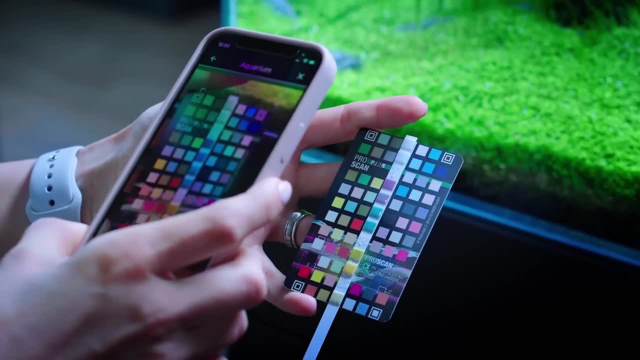 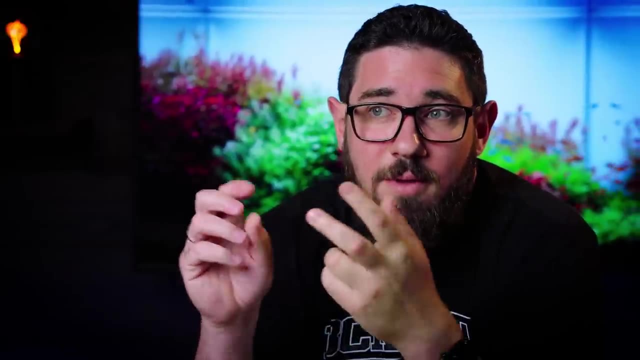 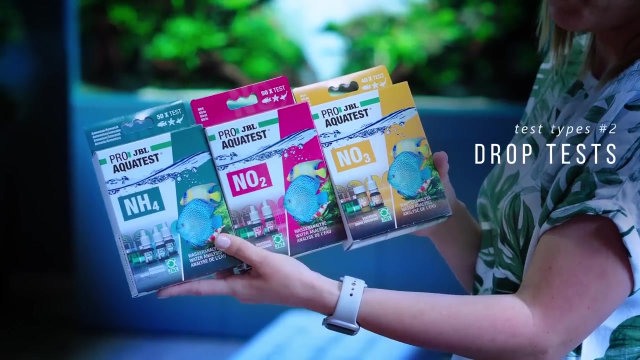 and then you can remove them. You can read of 5,, 6, 7 different water parameters. They're quick, they're insanely inaccurate, but they're good to see if something is extremely off where it should be. You should use drop tests to measure more accurately the same things. 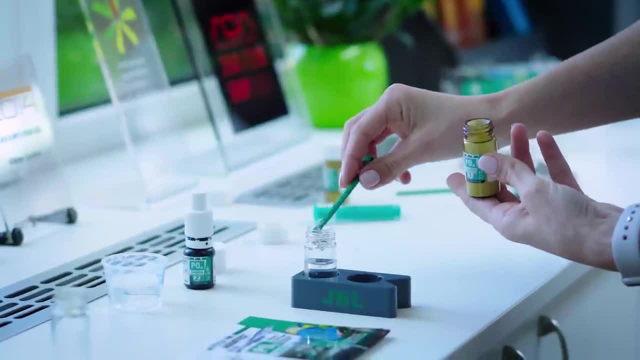 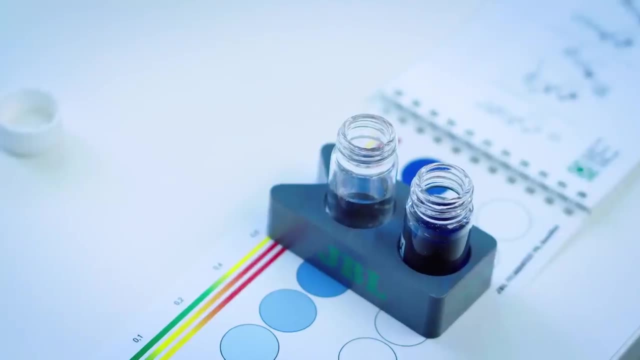 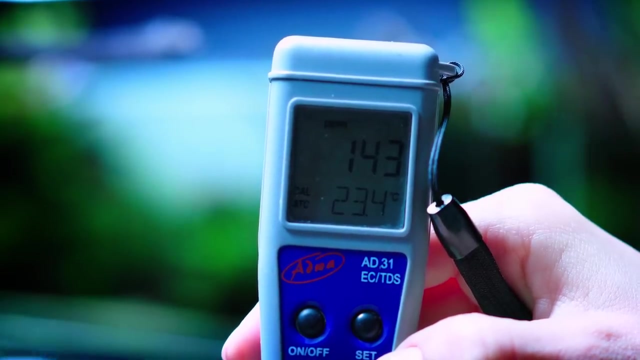 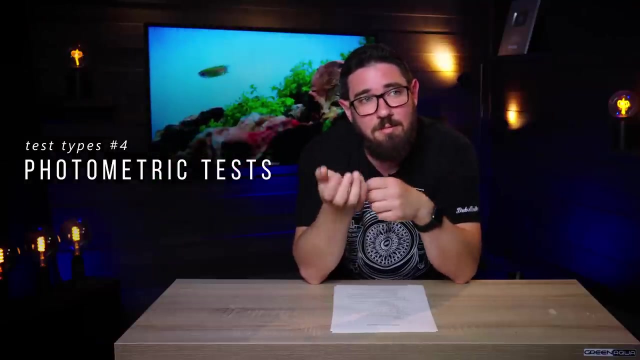 And also drop tests are available for a lot more different types of nutrients or elements in your water. Then we have the digital tests which mainly we use for pH and TDS. For really accurate stuff, you have photometric tests, which are basically drop tests read by a digital unit. 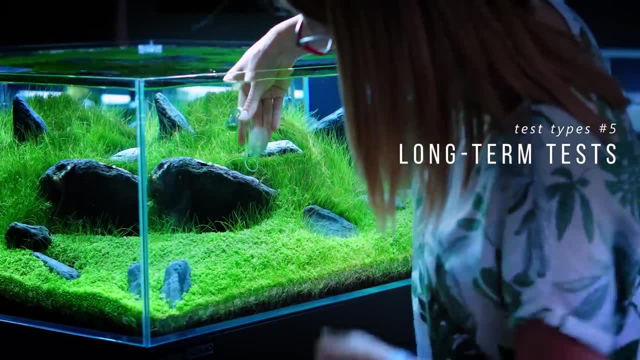 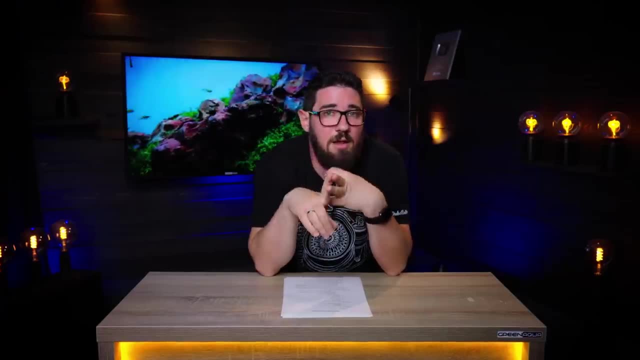 Also, there are some long-term tests like the drop checker in the aquariums, which measure our CO2 levels, and also like Seachem's ammonia alert and pH alert, which measure our pH levels, and also like Seachem's ammonia alert and pH alert. 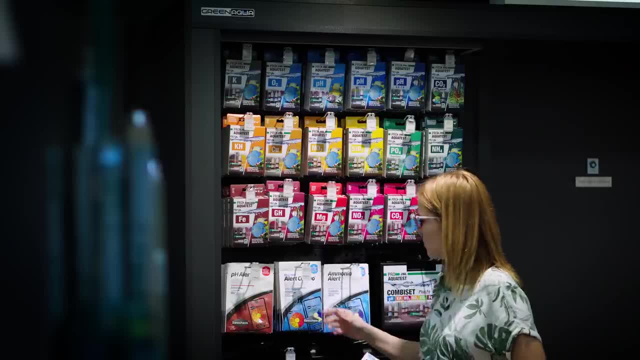 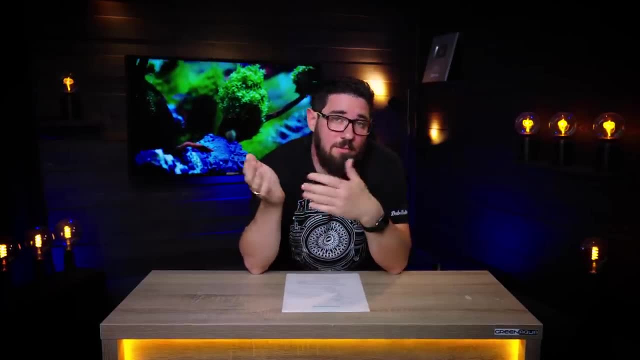 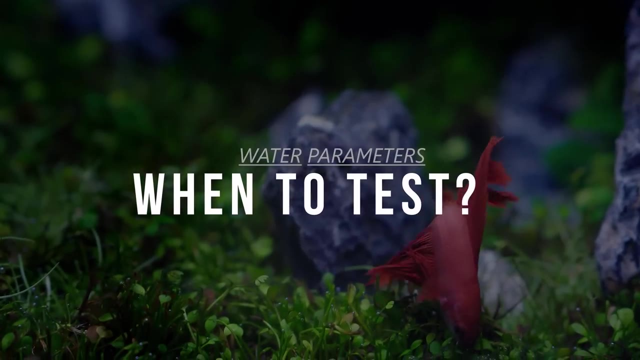 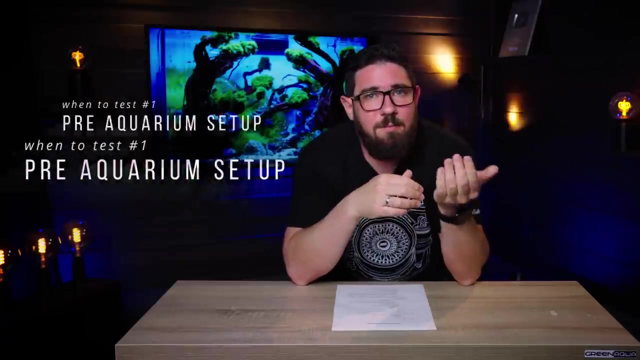 which you can use for up to 6 months or a year, always in the aquarium. So that was the how. Now, when and why do we test? First occasion would be: before you start your aquascaping journey, You should know what your local tap water is like. 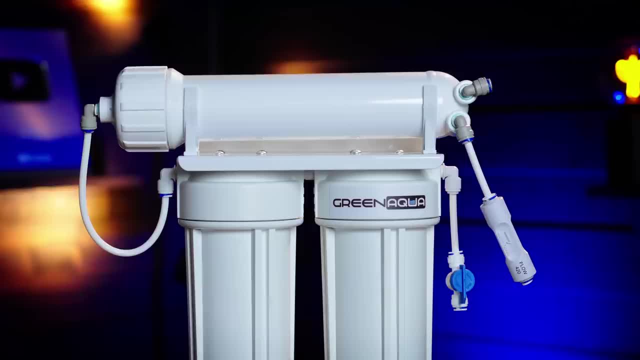 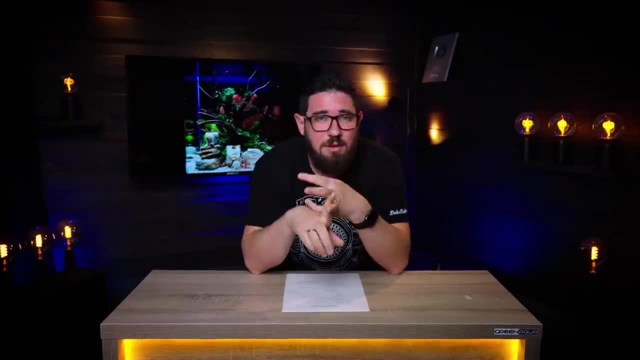 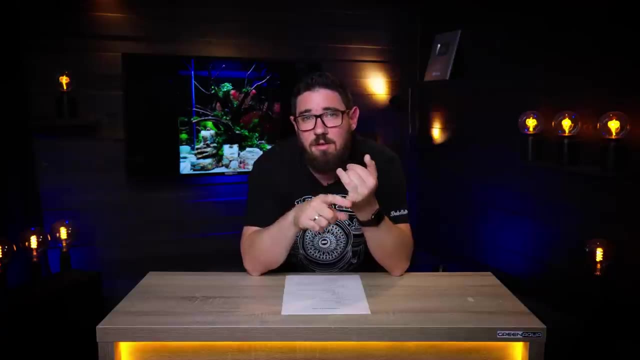 This is where you can decide if your tap water is going to be fine or you definitely need an RO system to even start out aquascaping. This is basically for GH, KH and pH of your tap water. These are important And also in some cases, like silicates level or iron levels. 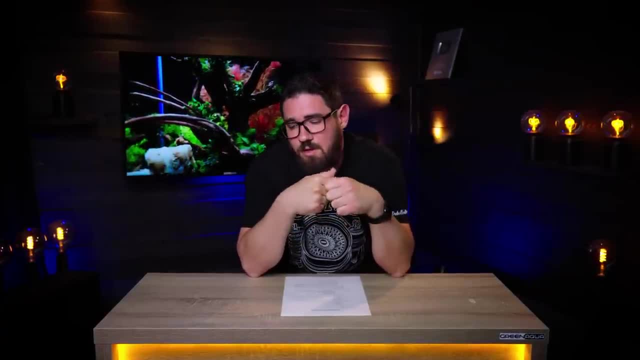 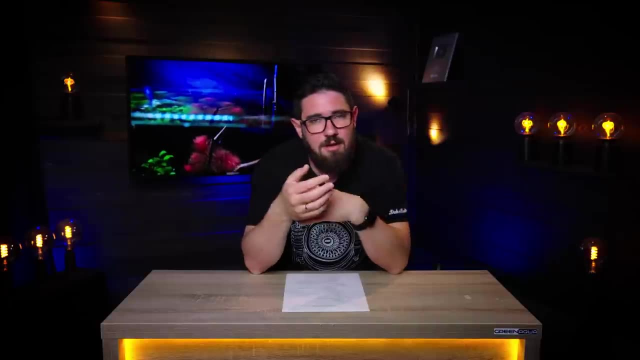 or even copper, can be really high in tap waters. So that's good to know upfront. You don't definitely need to buy tests to do this In most areas, at least in Hungary and, as far as I know, in a lot of places in the world. 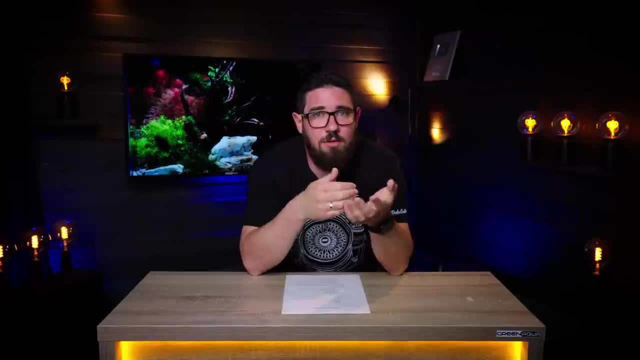 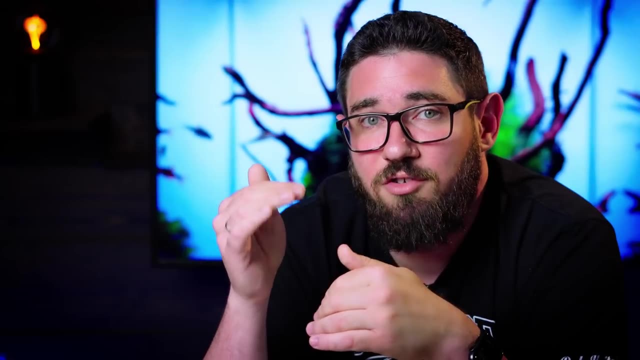 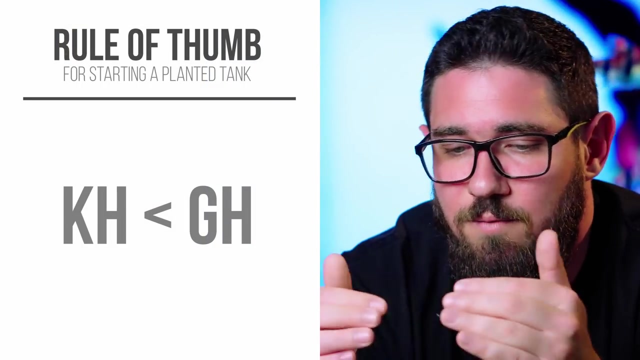 you can get this information from your local water supplier. The one thing that should be really putting you off when starting out: if KH is higher than GH, that's always a bad sign. KH should always be lower GH. It doesn't matter if we are talking about GH6 and KH2,. 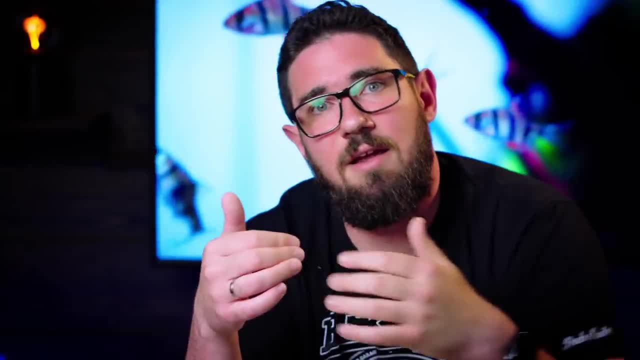 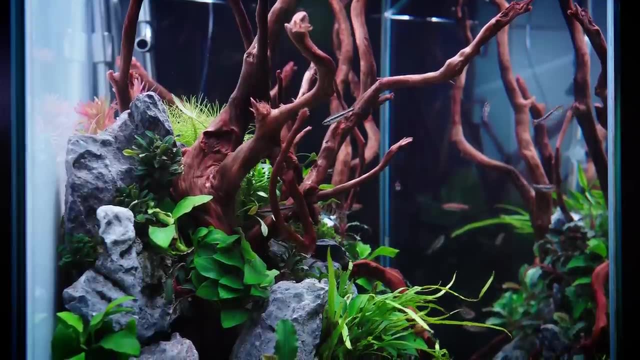 or we are talking about GH20 and KH16.. It's the same. There should be a small difference in between the two. If KH is really close or higher than GH, that's not going to be suitable for any kind of living things. It's not good for your plants, not good for your animals. The next step for testing would be after you set up your aquarium. After you set up the aquarium, it's worth doing a quick test, maybe one or two days later, to see how the water changes in the tank. 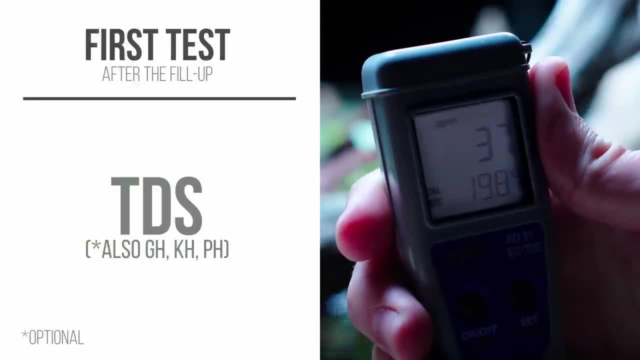 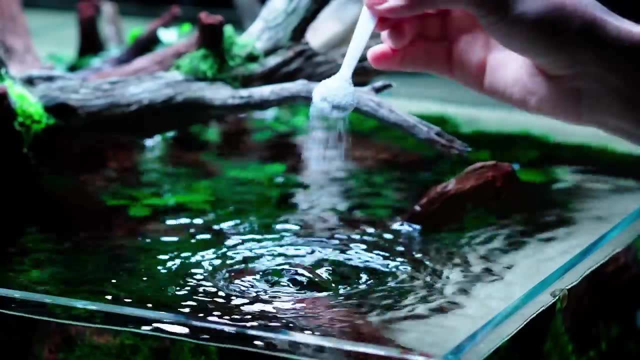 We obviously measure TDS right away after setting up, especially in case of using RO water. You need to remineralize the water even on the very first day. Some people think it's only needed once you add plants or fish or shrimps or whatever into your tank. 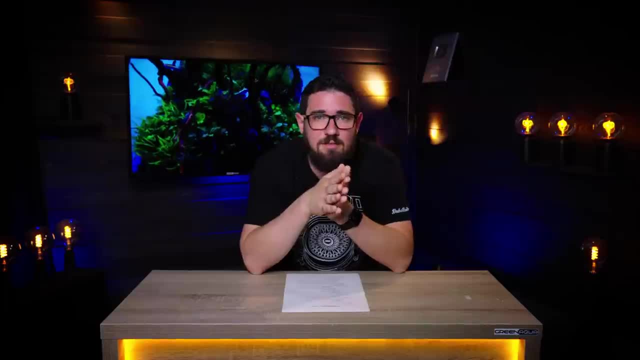 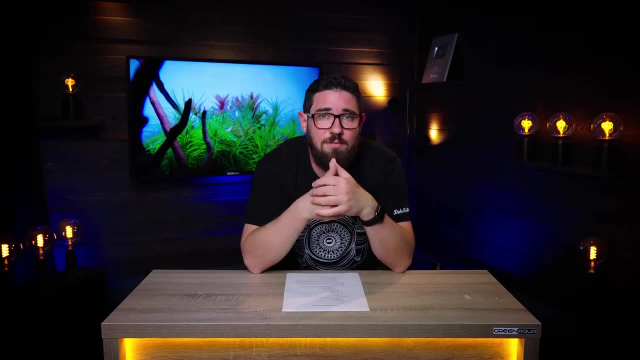 But actually it's important to have the TDS at least around 100 ppm from the very very beginning. Also, it's worth measuring your GH, KH and pH when starting out the aquarium, just to have some information of what's the base you are starting from. 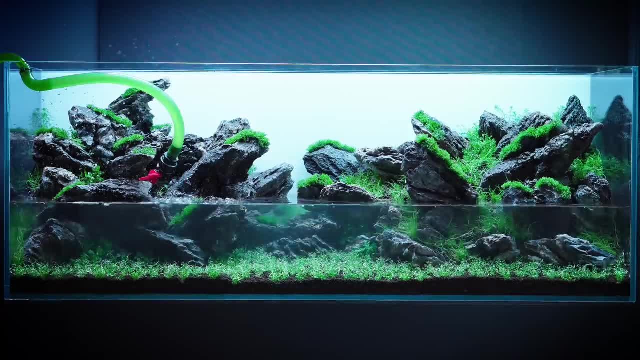 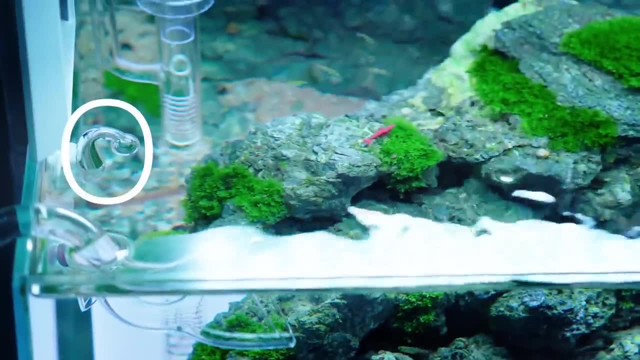 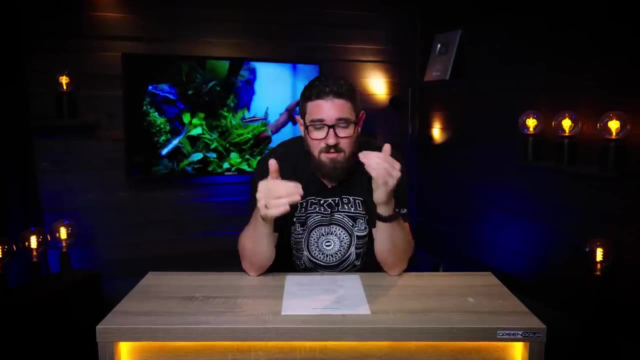 and how your filter media and the soil and everything else affects the water that you put into the tank. Also, after the initial setup, place your drop checker in the tank immediately if you are using a CO2 system, because this is the first few days when you can set it up precisely. And after that you don't really need to adjust CO2, if you find that perfect level. You know the lime green color in the drop checker that we are always chasing. Next time we would test is after two or three weeks of setup. 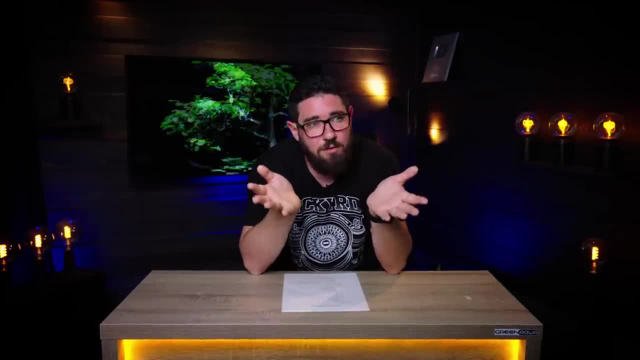 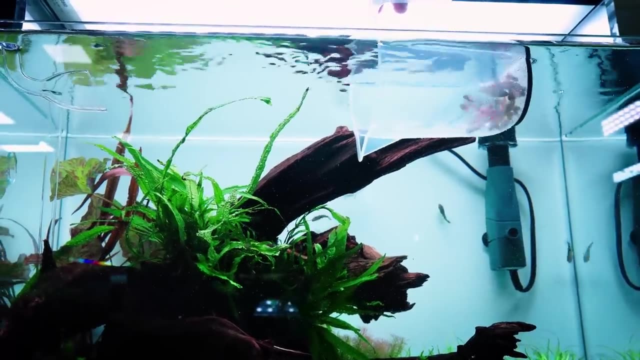 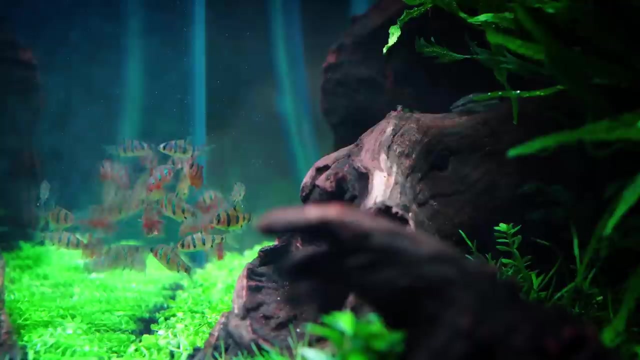 This should be the cycling period of a new tank. There's a lot of debate about this. We usually introduce fish and shrimps after two weeks, but we use huge filters. We use a lot of biological filter media. In most cases, we use filters that have been run. in already on another setup. So after two or three weeks you should measure ammonia nitrate and nitrate. If there is any ammonia or nitrate left in your water, don't put any fish into it. It's not ready. 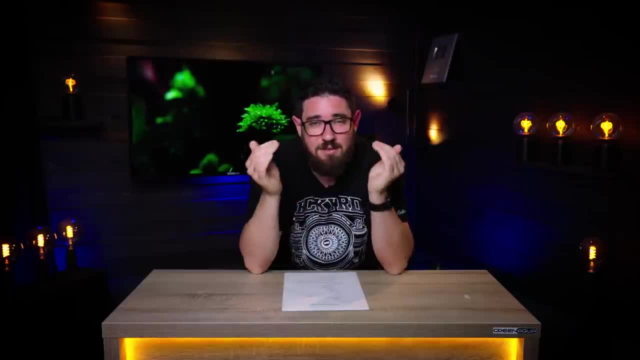 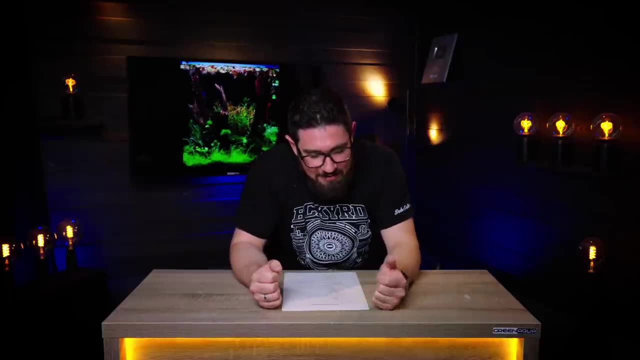 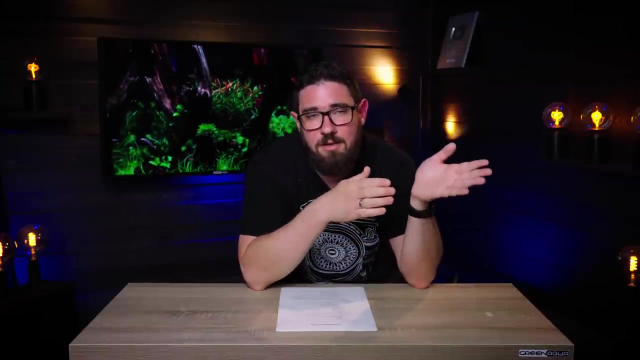 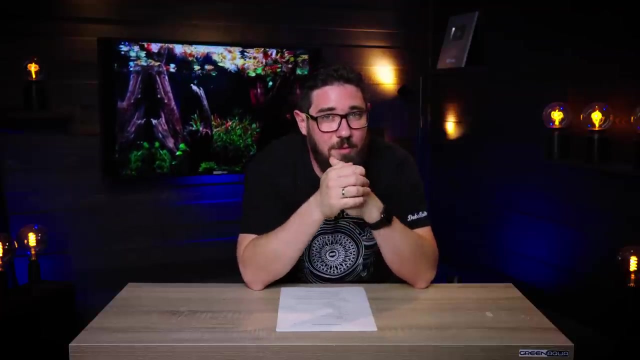 That's toxic for all animals, So you should wait. After this period comes the time when ideas start to divide and debating starts, Because everything I say from now on is our experience and how we usually do things. You might find different opinions online. 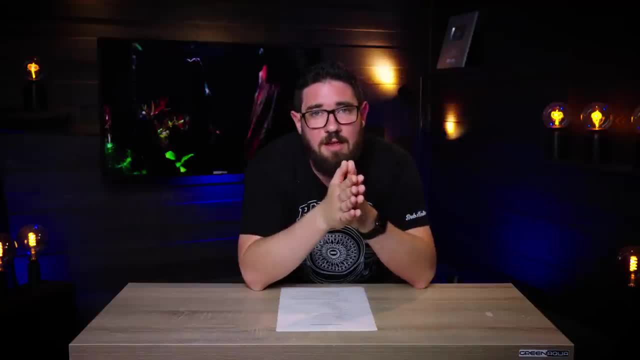 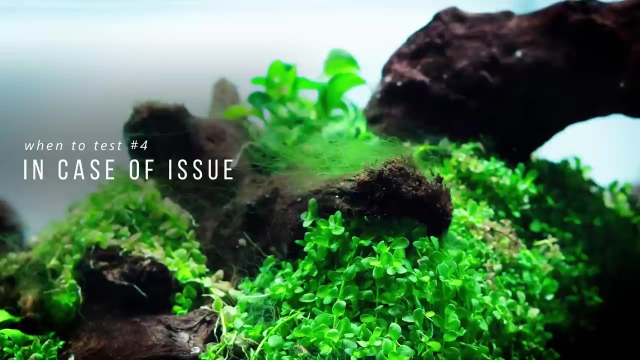 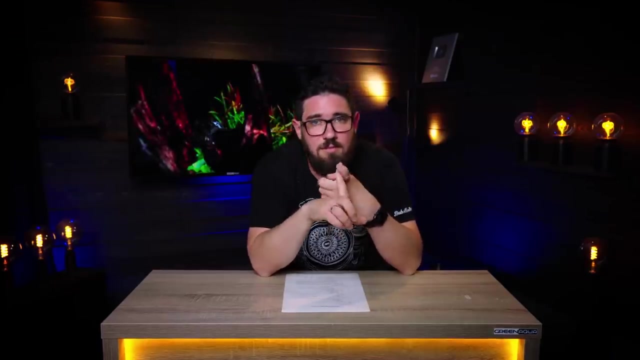 It's up to anyone. We usually say: don't test unless you definitely need it. We only do tests. when we have some issues like sudden die of shrimps or fish. We see something wrong with the plants or mainly algae issues. But even then, we usually just test a few things. Let's go in that order: Animals dying: The main things you should consider are anything that can be toxic. So, as we started in the cycling part- ammonia and nitrate- You should test those. But if you have your tank running for at least a month, there shouldn't be any. If you have any of those, then you have something seriously wrong with your tank. You don't have enough filtration. You don't do your water changes. 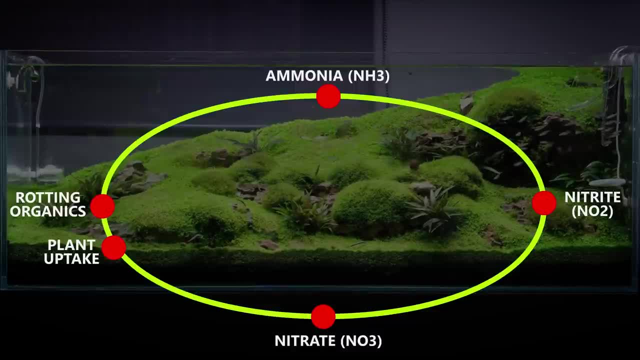 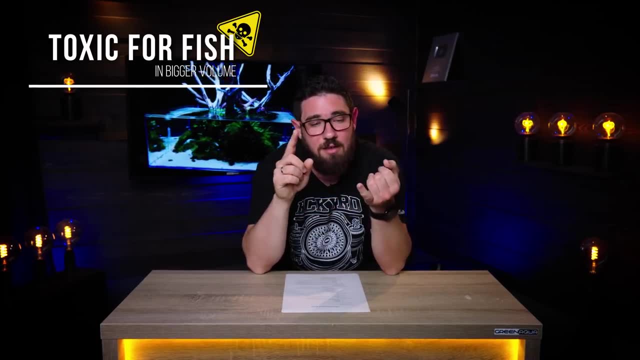 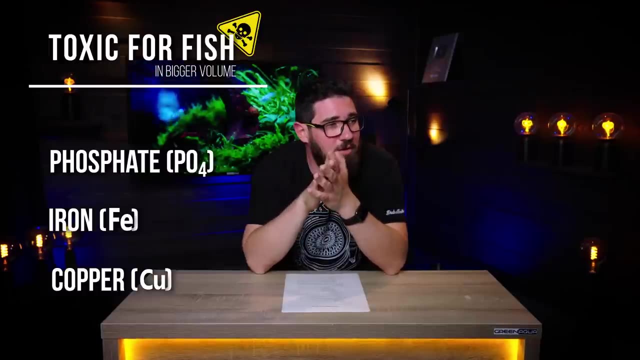 Your tank is overstocked, so your filter can't remove all the waste. That shouldn't be the first thing to think of In a planted tank. what can be too much and toxic is phosphates, iron and maybe copper. Copper is contained in most of the fertilizers. 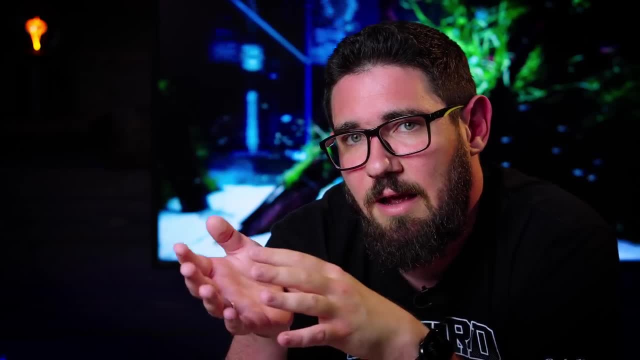 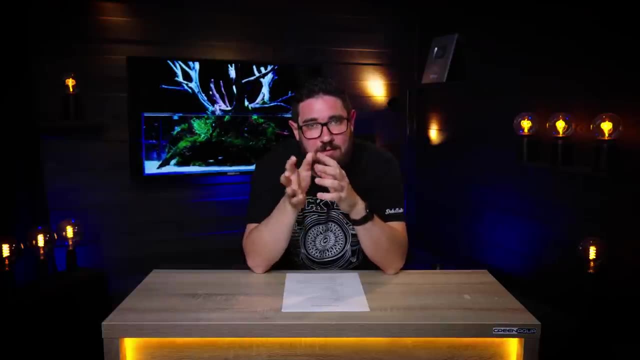 but still toxic for a lot of animals. So that's a tricky thing. In the fertilizers it's such a low amount. If you have measurable amounts of copper in your aquarium, that comes from somewhere. There's something in the tank. 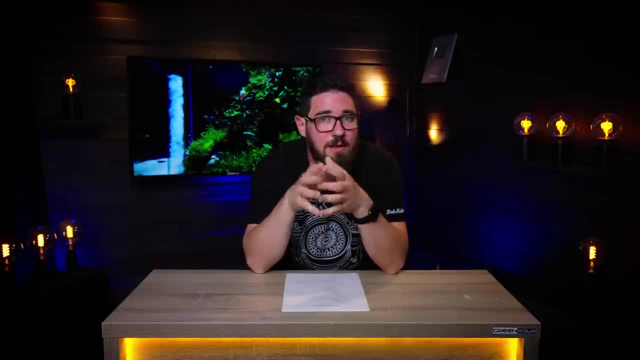 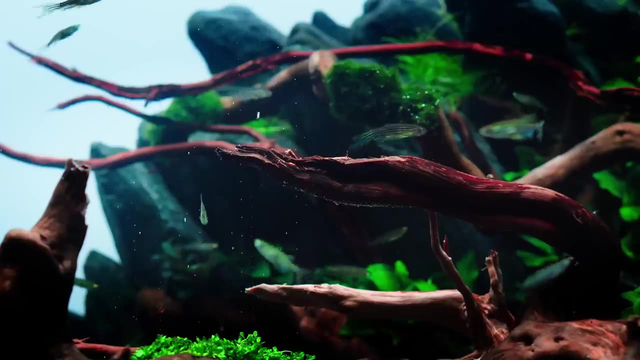 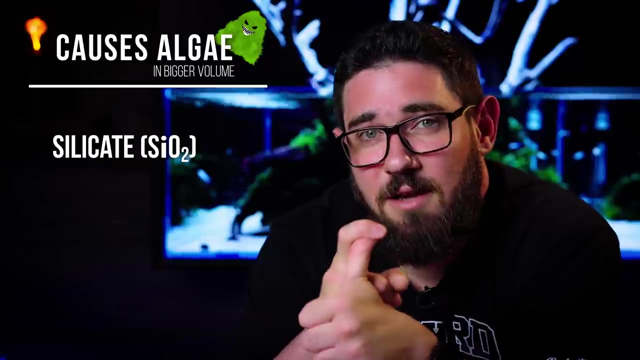 a piece of screw or your tap water has some copper in it or something like that. That's a problem. You need to work it out where it comes from. In case of algae issues, really common is high levels of silicates in the water. 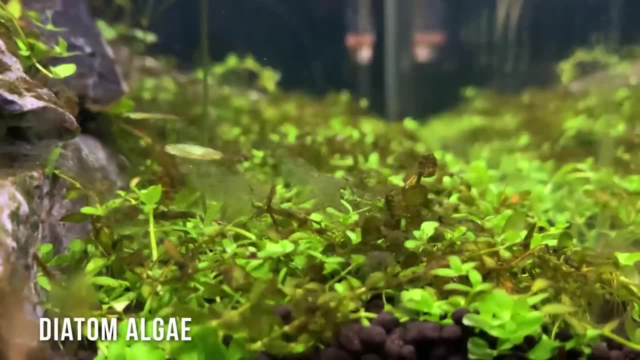 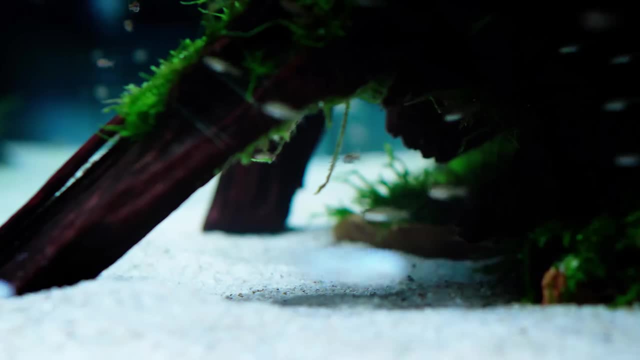 That can cause a lot of diatoms, especially when starting out the tank. This is a regular problem And in a lot of cases tap water contains high levels of silicates, And also if you use a lot of sand in the aquarium. 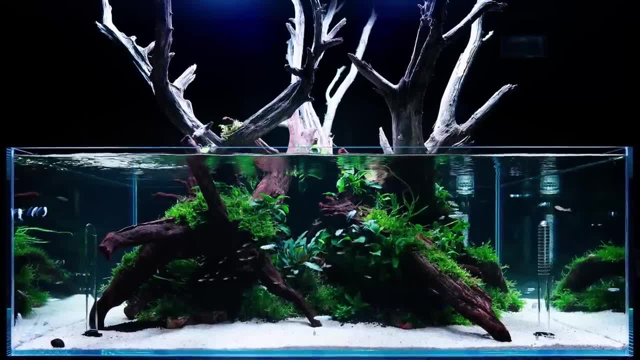 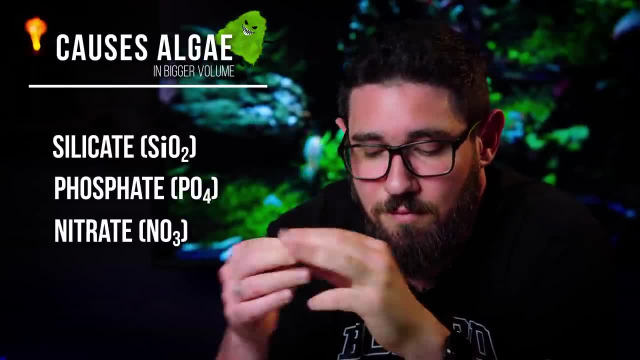 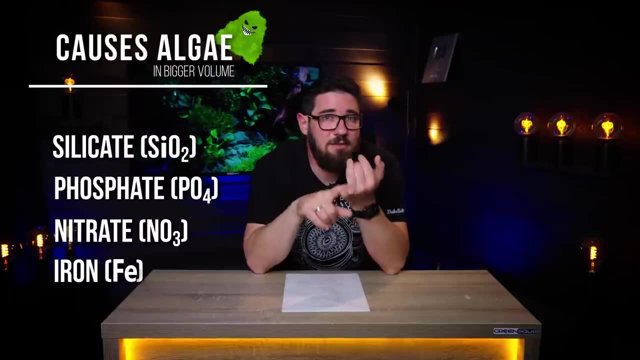 that can raise your silicate levels as well. In connection with algae, levels of phosphate and nitrate is also important, So I'm going to get to the levels we want later on. These are the things we measure, And also iron: High levels of iron in a tank. 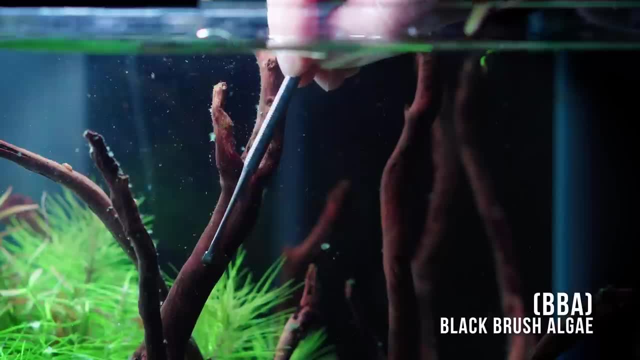 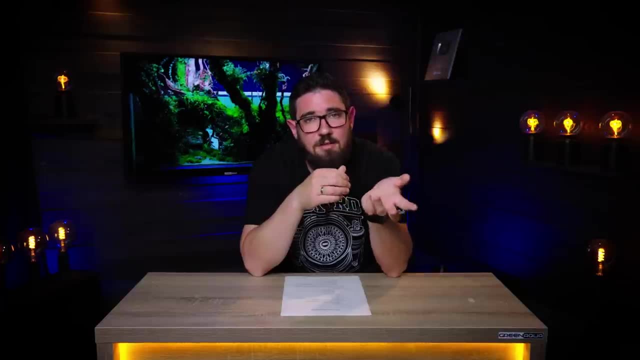 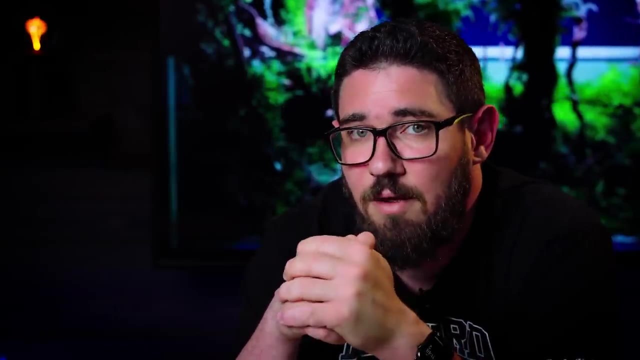 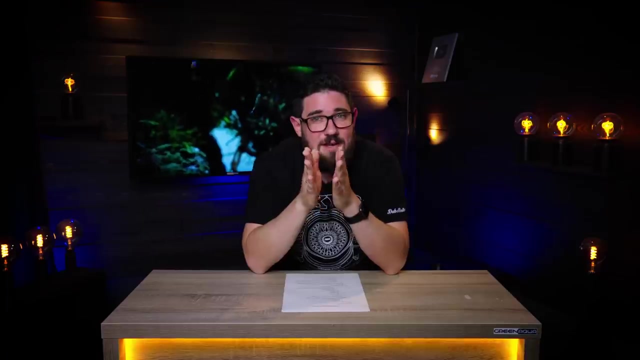 can really help BBA to grow in the aquarium. It doesn't come from overdosing iron, but once it gets into your tank, high levels of iron helps it to grow And, yeah, it can get out of hand quite quickly. It's really, really difficult to say what to test. 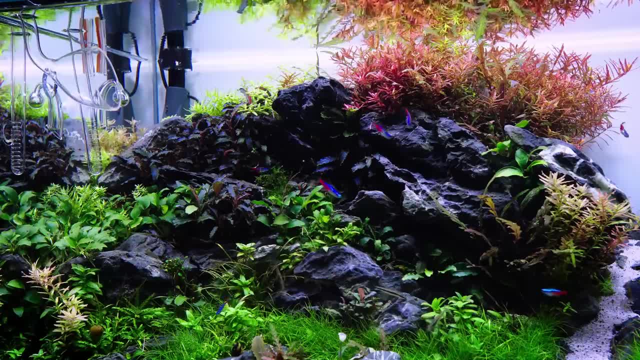 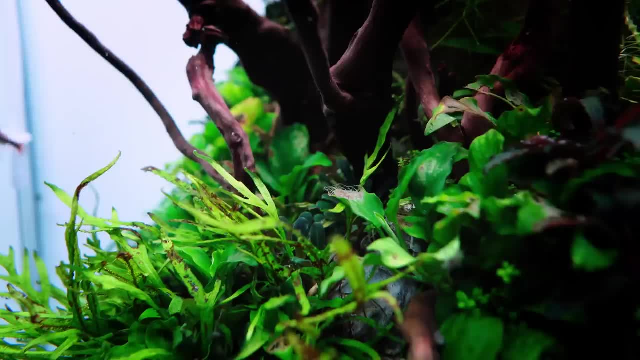 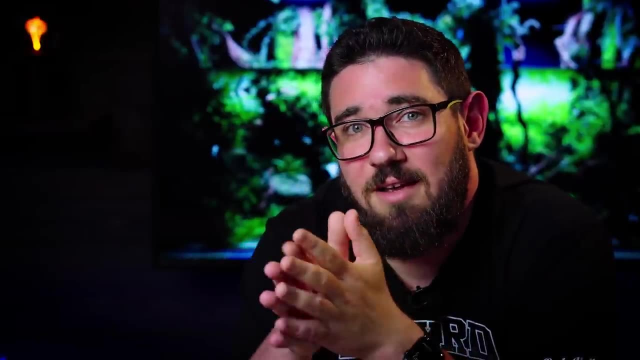 when you have plant problems, When you see your leaves curling or there's not enough color in the plants or they turn yellow, they drop their leaves. Most people think about nutrient deficiency right away, which is, in 90% of the cases, wrong. 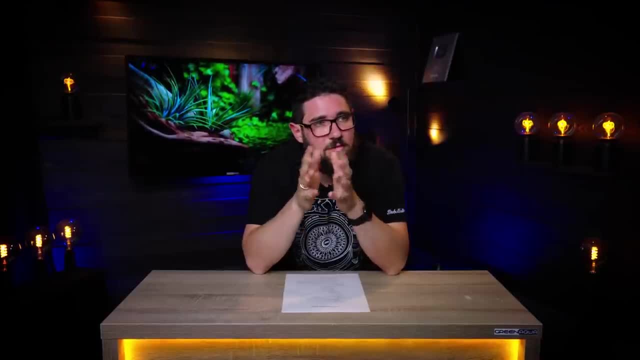 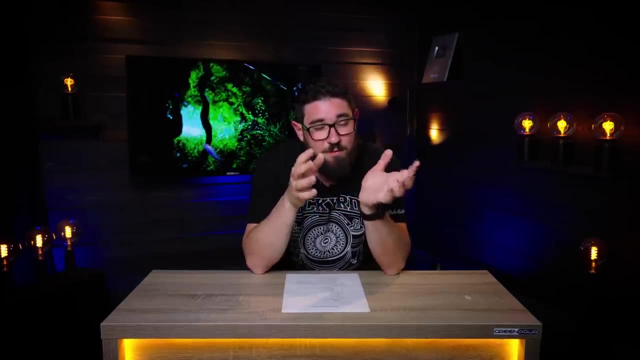 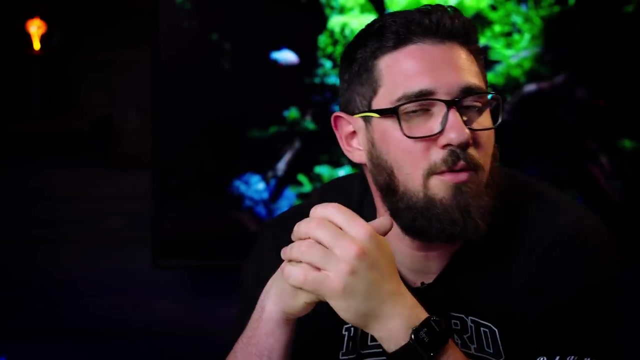 It's more about the levels of CO2 in your tank, the lighting of your tank, the maintenance routine. You can find deficiency charts online for plants, which says that if you see this, then measure potassium And probably that's going to be the problem. 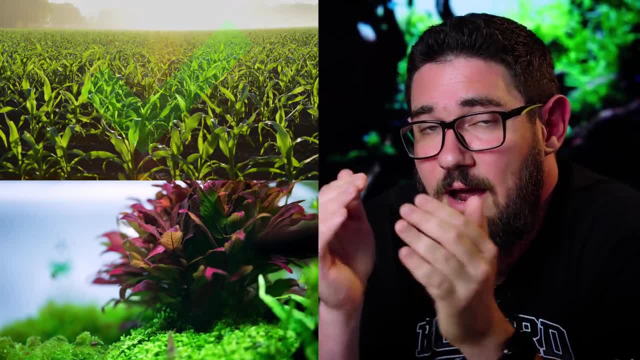 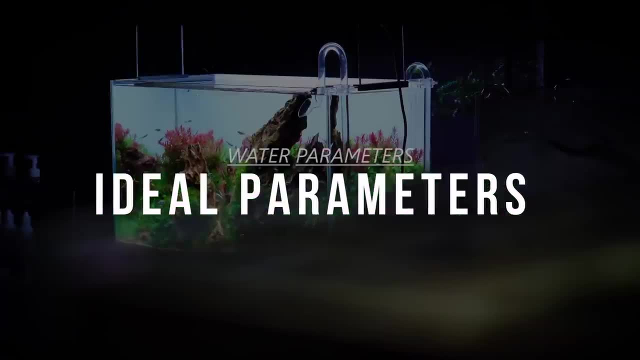 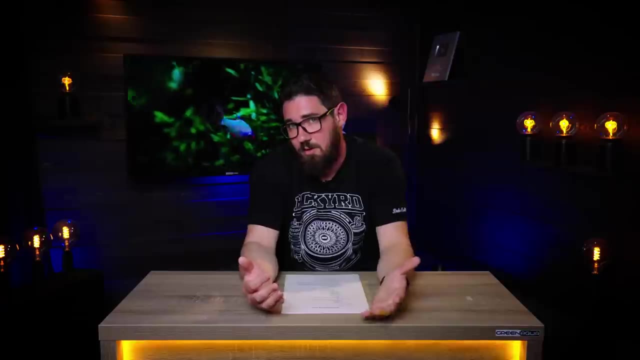 The issue with these charts is that they are made for agricultural plants. They have nothing to do with aquatic plants. What are the numbers we're aiming for? Well, let's go with the stuff that's common in every tank. I'm talking about tanks with RO water. 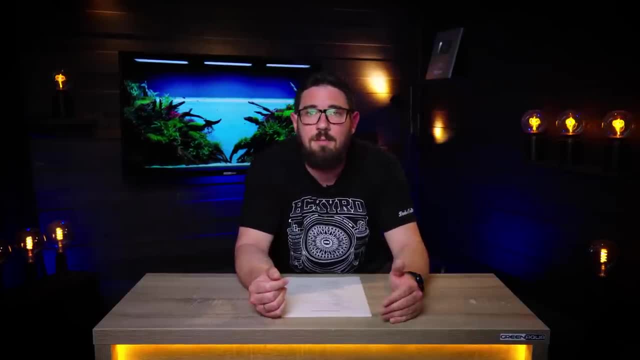 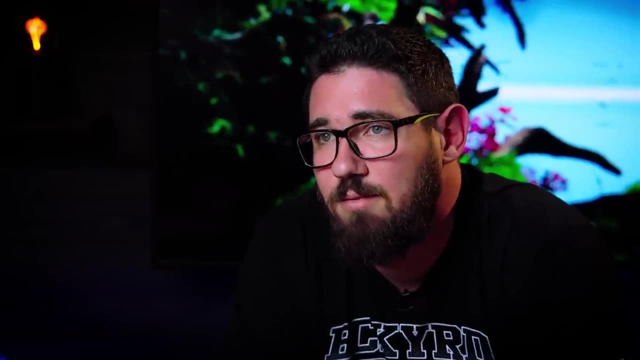 because in tap water you can't really do anything with the main stuff. So GH, KH, TDS, you can't really change it. I mean you can raise them, but that's not going to help in any way. So if you have tap water, 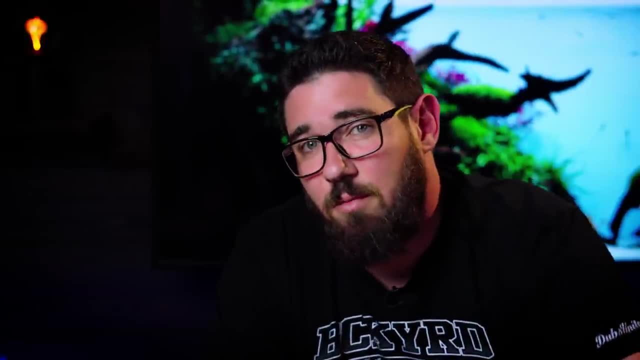 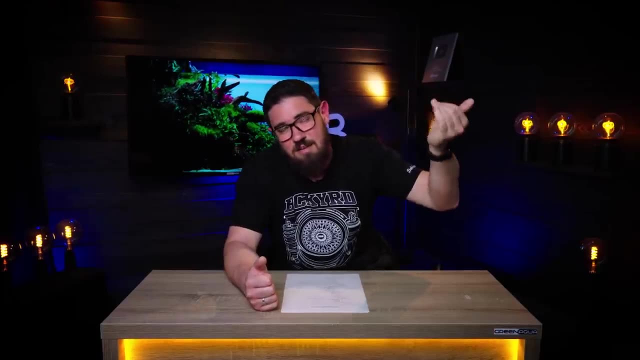 you deal with what you have. The only thing that can be a real problem is the water is too hard or, as I mentioned, if KH is higher than GH. In that case you could raise GH even in tap water to flip it around. 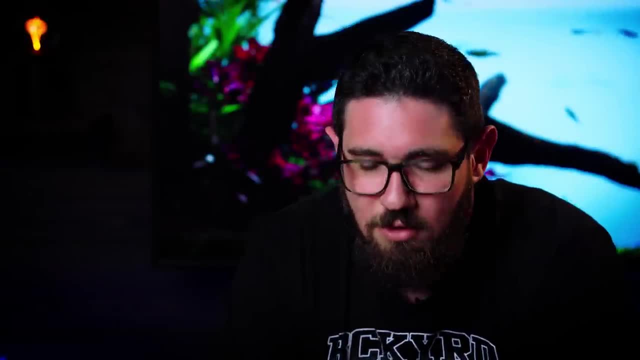 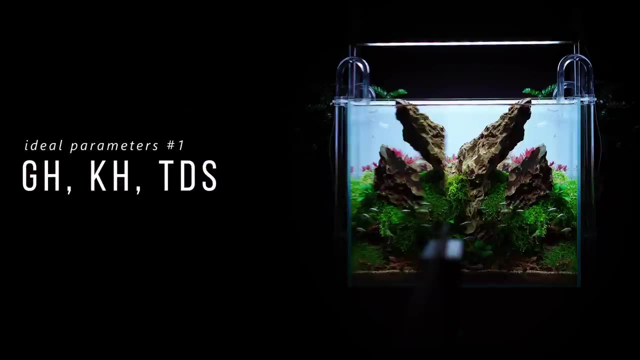 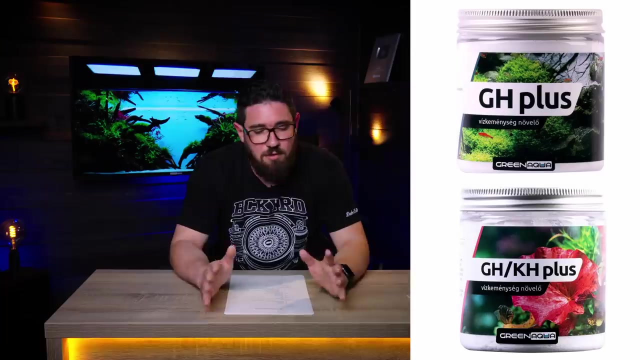 but then you're going to have really hard water. So in those cases I would recommend switch to RO water. So when you set up the tank with RO, you should use a remineralizer, either GH Plus or GH KH Plus. We talk about this a lot. 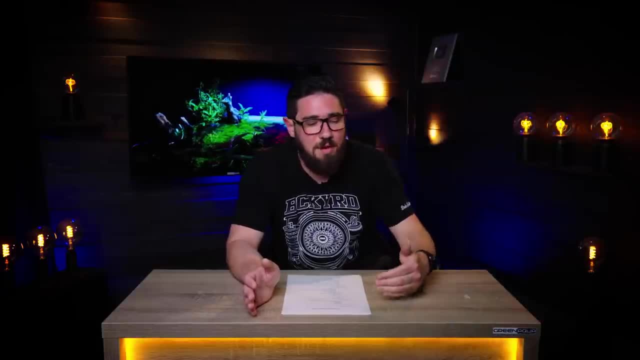 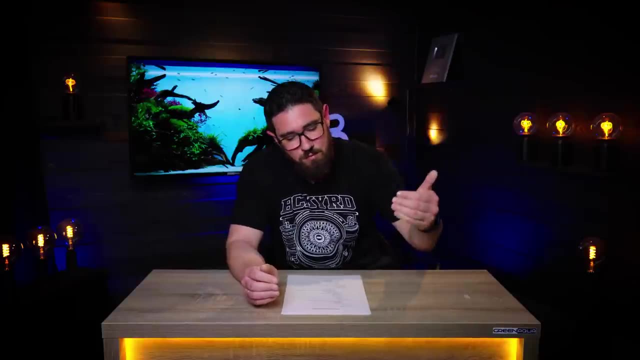 It depends on what's in the tank. If you have anything that's going to raise KH as well, then you only need to add GH Plus. So, for example, if you have serious stones which have thin lines of limestone in it, 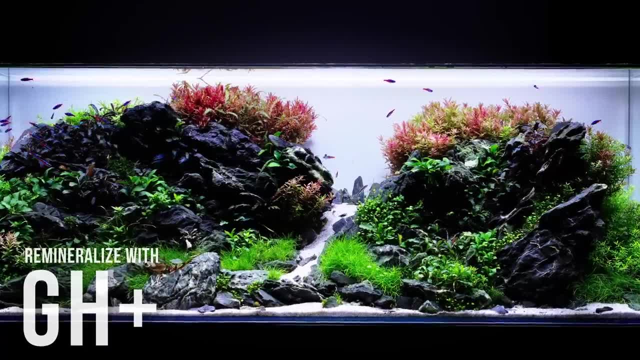 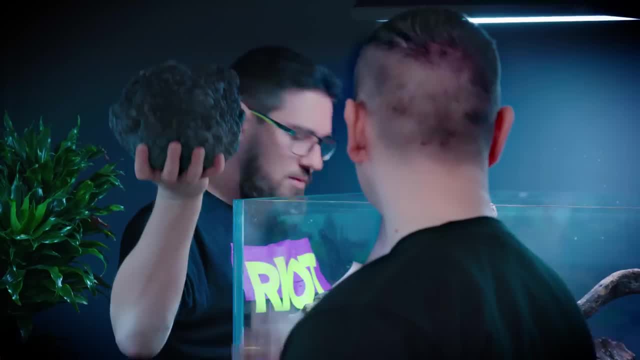 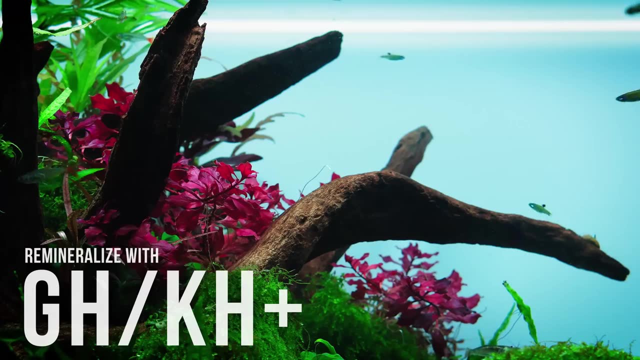 that's going to raise your KH on its own. You only need to use GH Booster. If you have a tank running with lava stones and iron wood which don't really affect GH or KH, then you should use GH KH Booster to have that very low amount of KH that's needed. 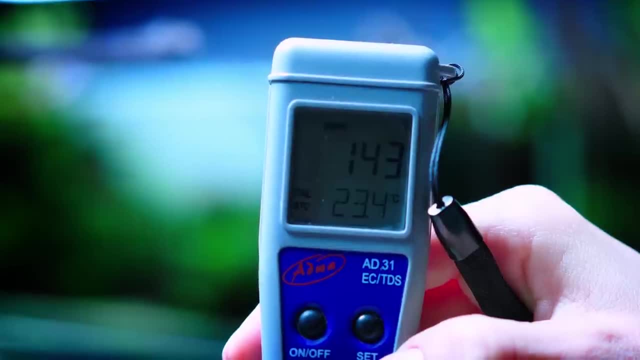 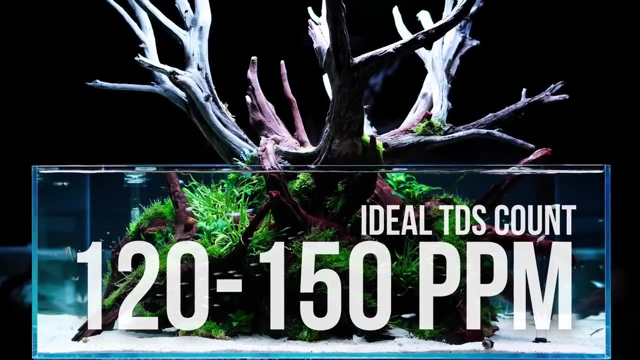 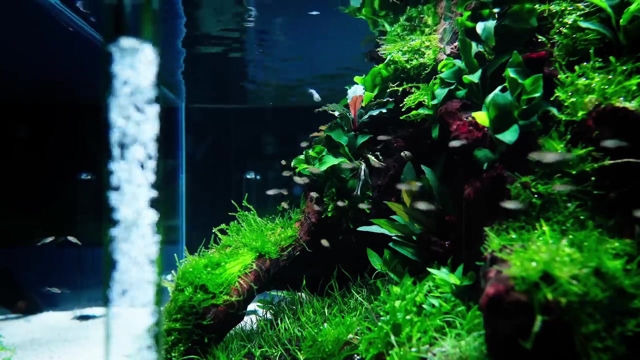 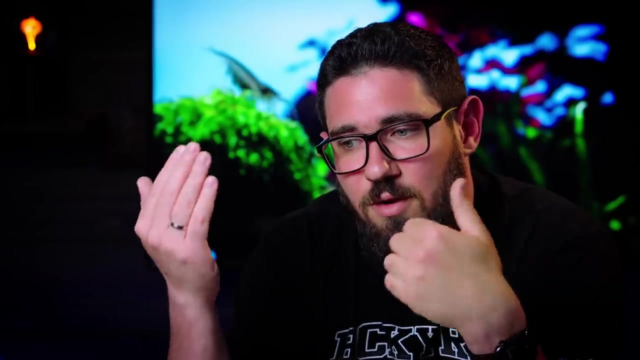 So TDS? You aim for a level of 120-150 ppm in TDS. TDS is all the salts dissolved in your water. You can raise TDS without affecting GH or KH, So that's why you shouldn't mix these. 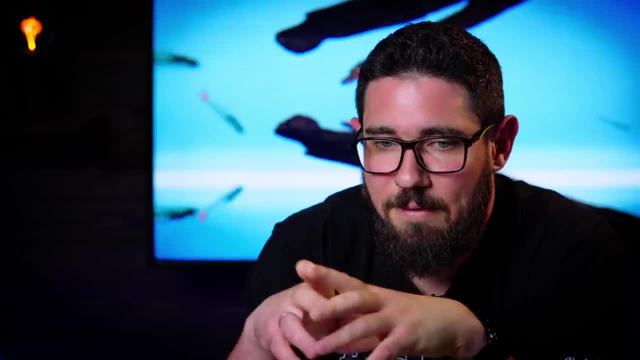 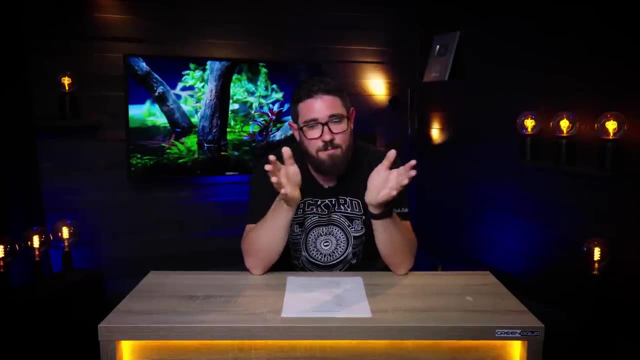 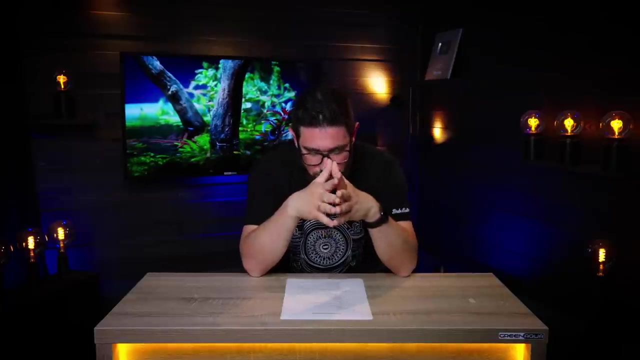 A lot of people think that these things are interchangeable and you can calculate one from the other. That's wrong. You decide You go by TDS or you go by GH and KH and measure them separately. If you go by TDS and the tank is working, fine. 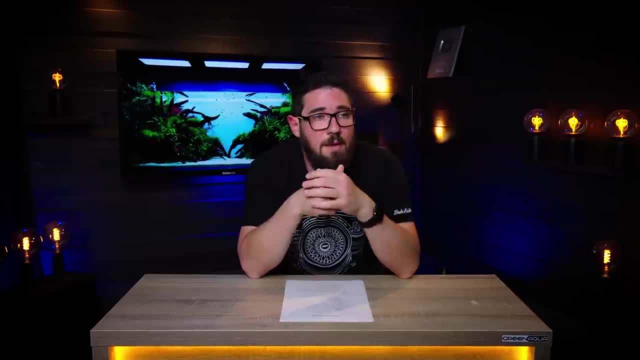 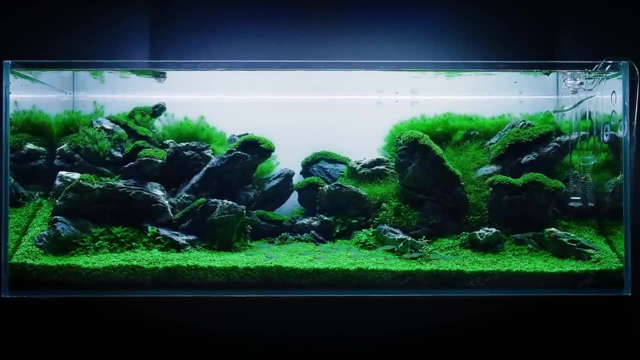 then 120-150 is a starting point for the week. It's normal. if this raises during the week, You don't need to keep it at 120-150.. You can't do anything about it. For example, again with Serious Stones. 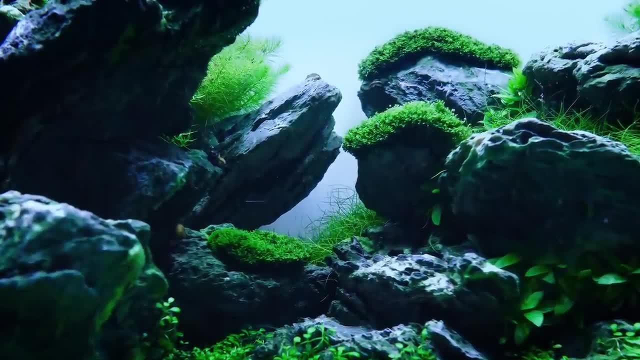 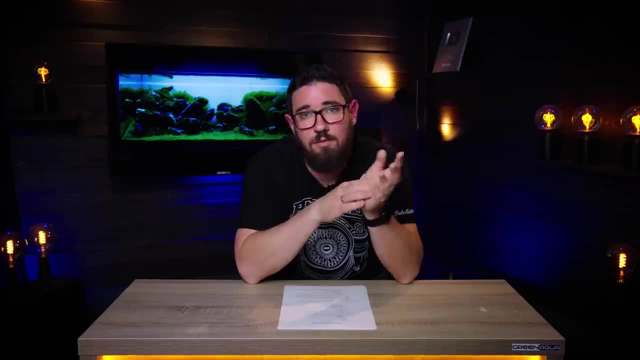 it's gonna go up even over 200 by the end of the week. That's fine. It's still a lot softer than what your tap water probably is, So perfectly fine If you're going the other way and you're measuring GH. what you should be having in your tank is GH 3-6.. Somewhere in there would be the sweet spot. You can narrow that down to 4-5. If you really want to be precise. But 3-6 is fine. 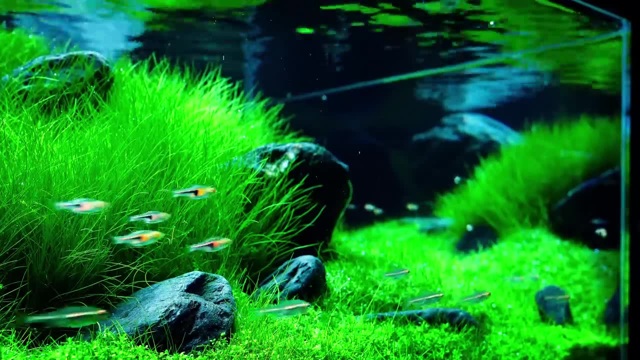 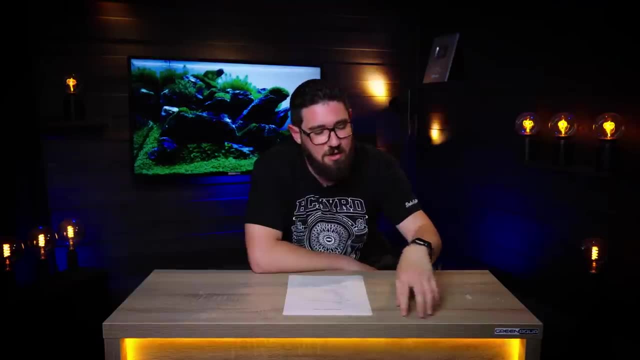 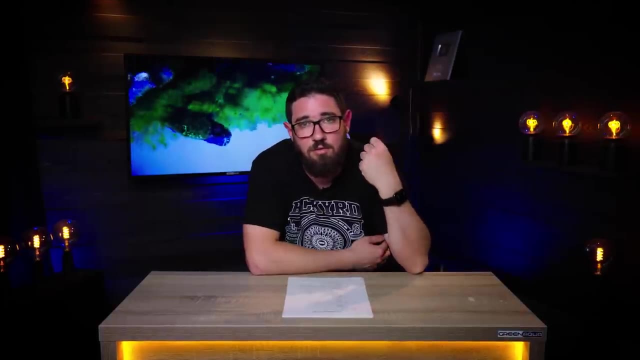 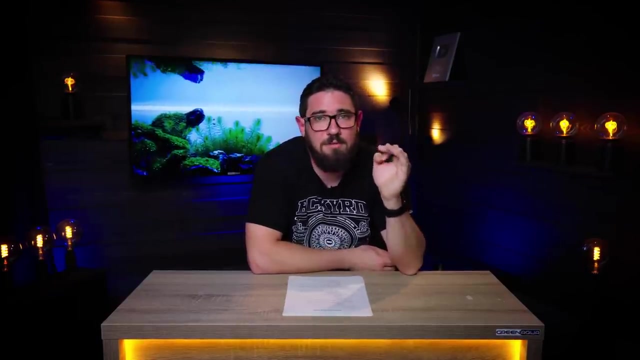 For that you need KH around 1.. GH is important, for example, for your shrimps. In GH is all the salts that are in connection with the shrimp's ability to create a new shell. Same goes for snails. On the other hand, KH: its only purpose is. buffering pH. The higher the number of KH is, the less CO2 can drop your pH. If you have KH 1 and you turn on CO2, pH is gonna lower quite quickly. Still fine, It's not dangerously quick, but it's measurably quick. If you have KH 10 and you start your CO2, the drop will be much, much slower in your pH. That's the only difference. KH 1 is usually maintained by most active soils- A good indication of low pH, especially in starting a new tank. 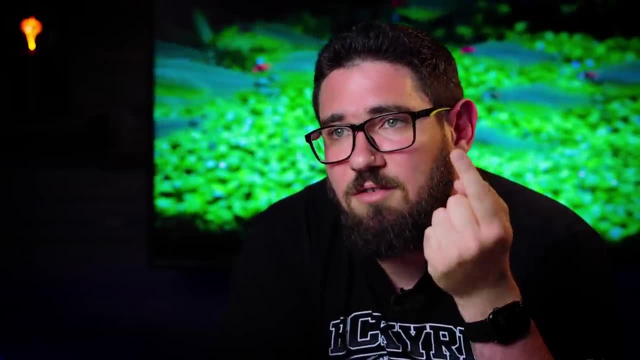 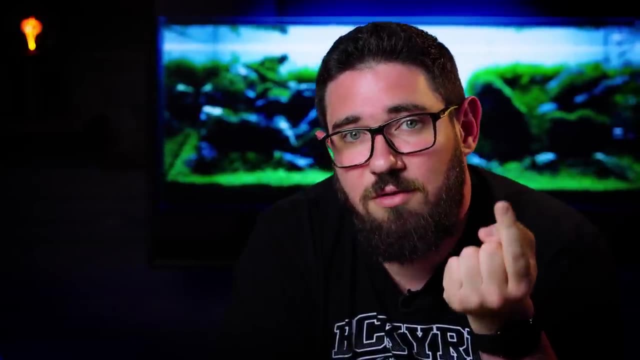 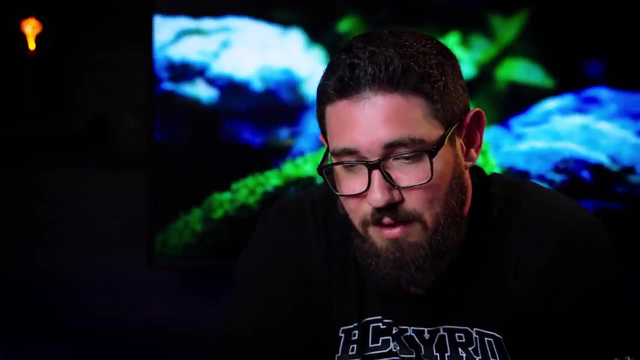 is plant melting. That's the only time I would suggest you measure KH, because that might indicate that KH is 0 and your pH is fluctuating crazy during the day because there is no buffering of pH in the tank. But that's it. 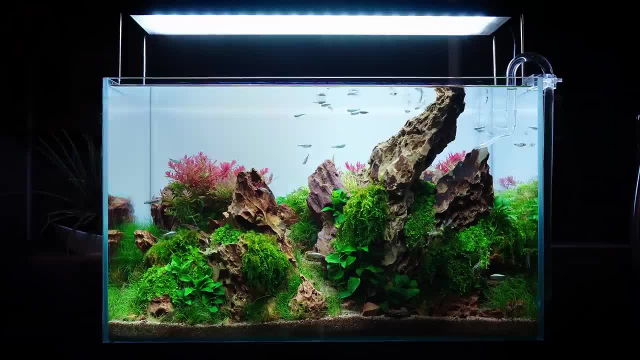 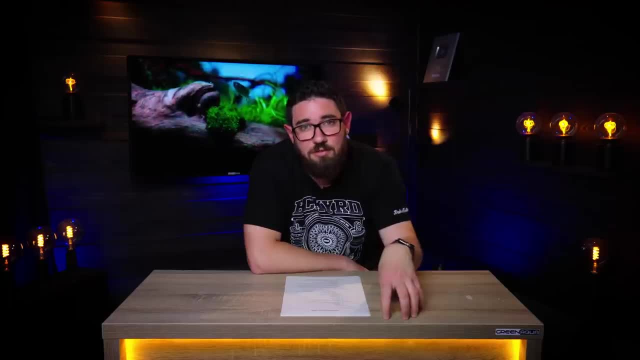 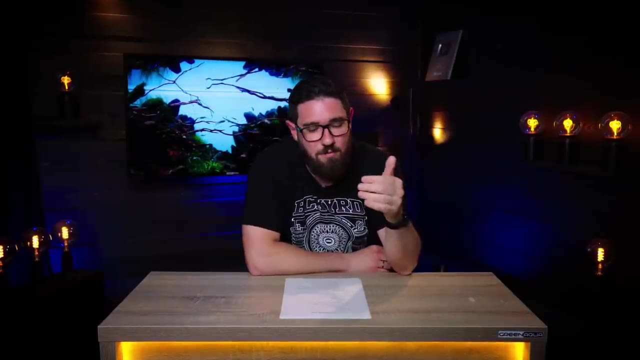 Any other case, I wouldn't even bother measuring KH. And then we arrive to pH. I mentioned crazy swings in pH is wrong, but what is crazy Well in nature? one full point of pH swing during 24 hours is perfectly fine. 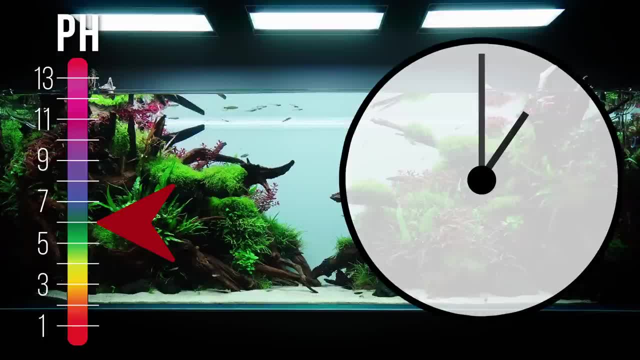 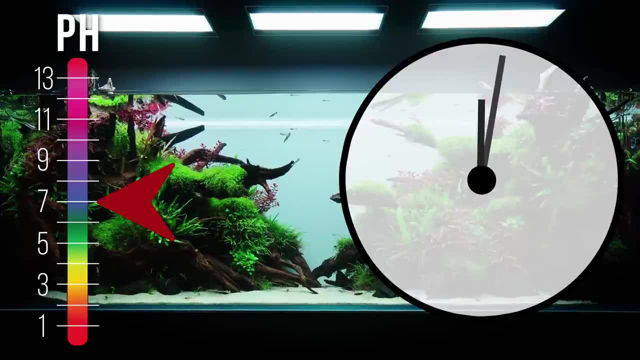 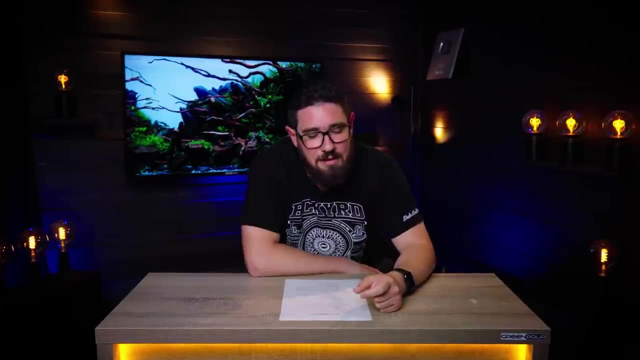 If your tank is pH 6 in the middle of the day, with CO2 running and everything, and then at midnight it's pH 7,, fine, don't worry about it. If it goes more than one full point during the day, that can be a problem. 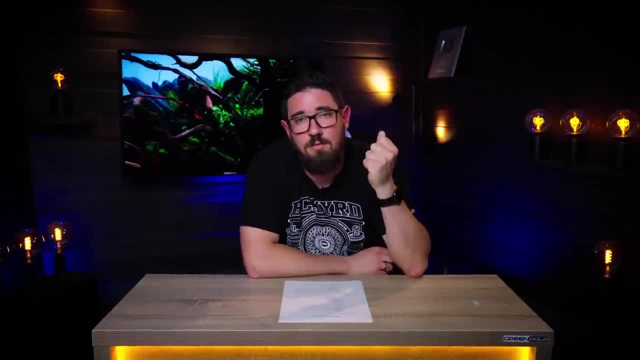 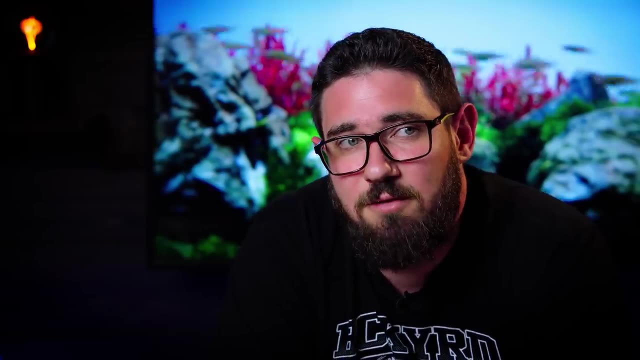 That means, for example, you don't have any KH in your water, which would buffer the pH levels, and it can go into crazy swings. What the pH level should be, that's more difficult to say With tap water, your pH in the aquarium. 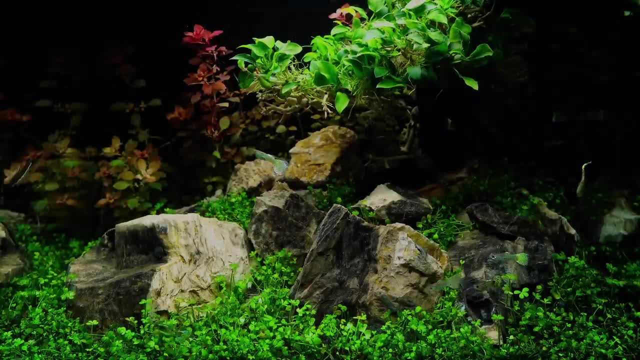 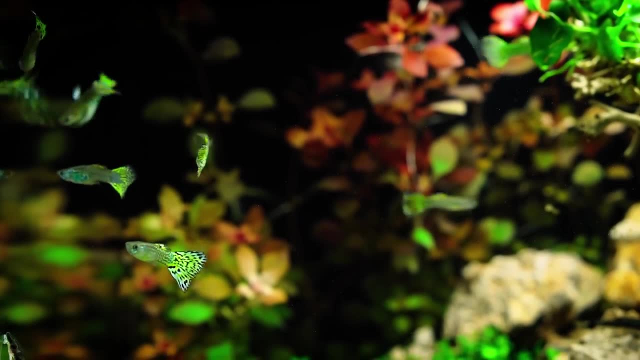 considering active soil, CO2, whatever your pH should be between 6 and 7.5.. So that's quite a wide range. With tap water it's actually really difficult to reach 6.. So when you put in tap water, 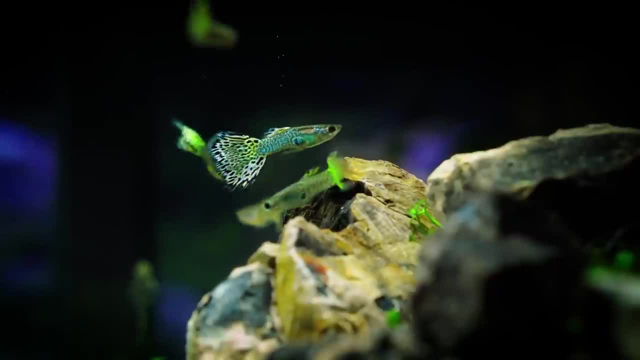 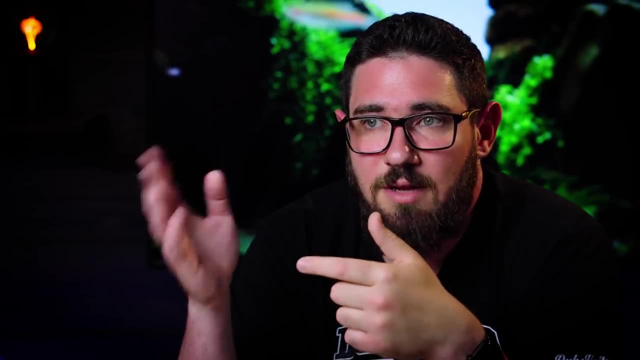 and, for example, your tap water is 7.5 to start with, You put it in the aquarium. your soil is going to lower it. You add CO2, that's going to lower it. Maybe your filter media, because there are kinds. 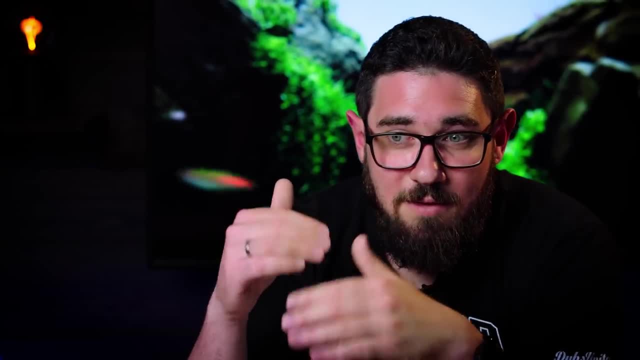 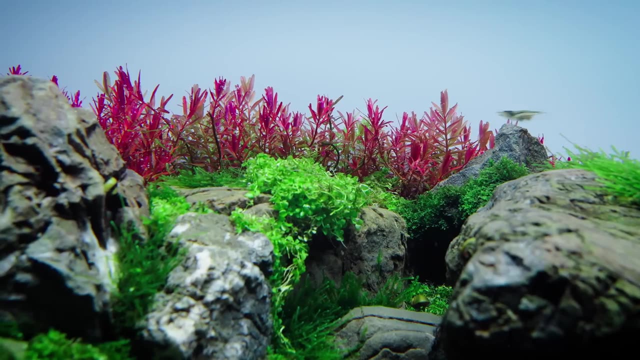 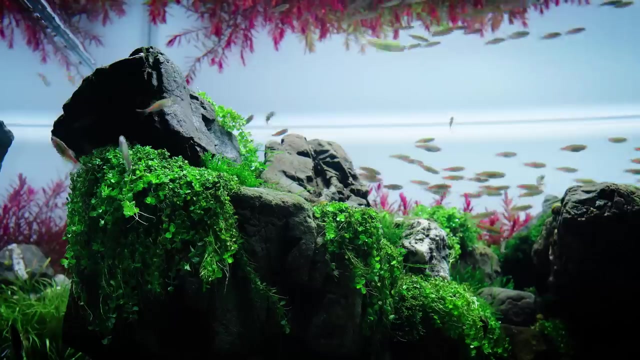 of things that can affect pH as well. Even all this wouldn't pull it down to 6. Probably, But anywhere between 6 and 7.5, it's fine. For RO water it's already softer, obviously. That's why it already has a lower pH. 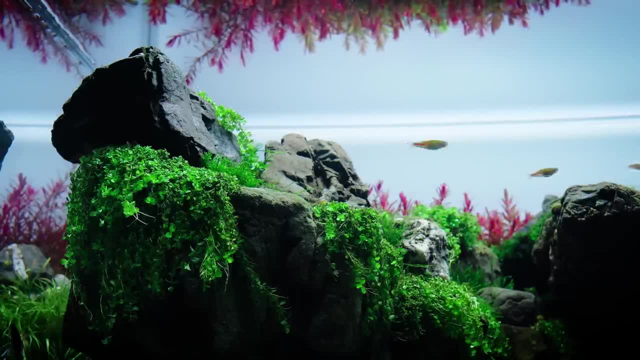 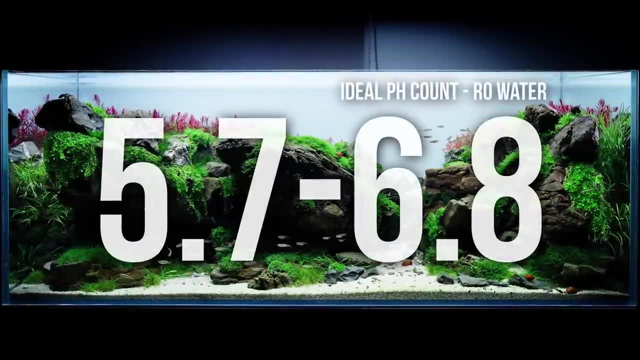 than tap water. So when you measure it in your tank with TDS set up and everything, you should read anywhere between 5.7 and 6.8.. Probably that's the area where it could be And here is a big misconception. A lot of people say that if your pH drops below 6, then your filter bacteria will die. That's not true. In a lot of places in nature there are rivers with pH 4 and 5. They work. Obviously there is some bacteria. They've been working for thousands or millions of years, So probably nature knows best. The thing that bacteria can't survive is a very quick drop of pH. Another thing where pH matters is keeping the fertilizers stable, So all kinds of nutrient, chalates. the form that nutrients are stored in. they have a range of pH where they are stable, But this is mostly important for storage. when they are in the bottle itself, Most of them are kept between 6 and 7 pH. They are quite normal, easy to reach. and they are stable for years. If you have a tank running with pH 5.5 and you add your fertilizer, it won't have any issues. It dilutes in the water quite quickly. Your plant is going to take it up nicely. 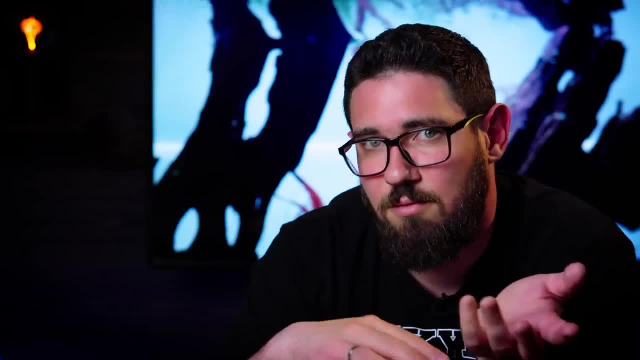 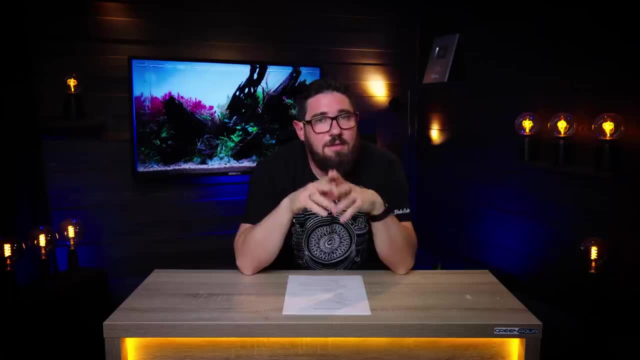 If you would put a fertilizer in pH 2, that would be an issue. But if you have pH 2, then don't touch that water because you're going to get burnt In some cases, when keeping a more stable pH is important, 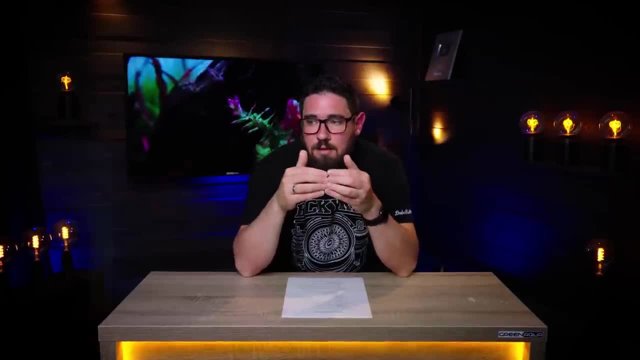 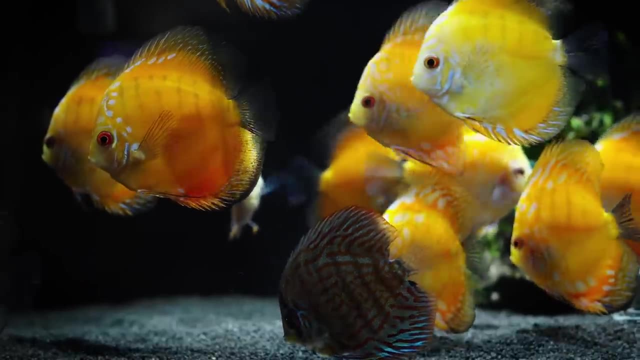 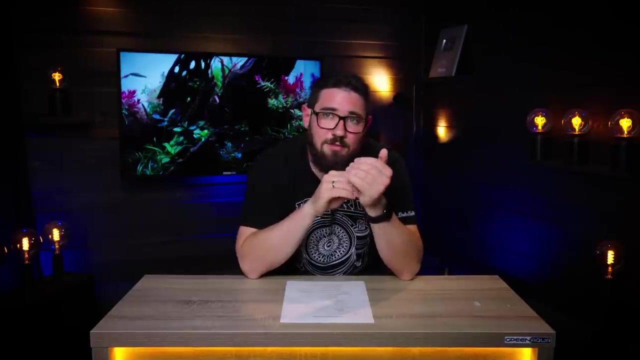 some animals don't like the one full stop swing that I mentioned earlier. So, for example, discus fish a lot of shrimps. they're really affected by high swings. In those cases it's recommended to add CO2, not by a timer. 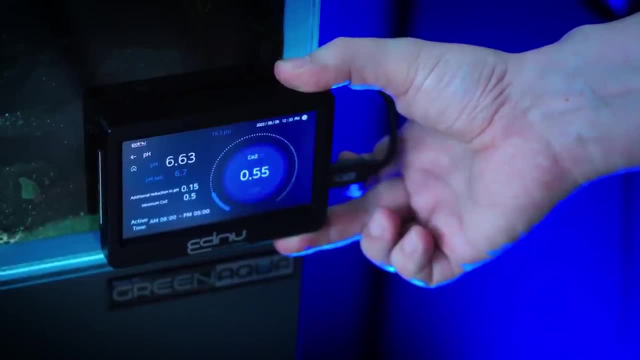 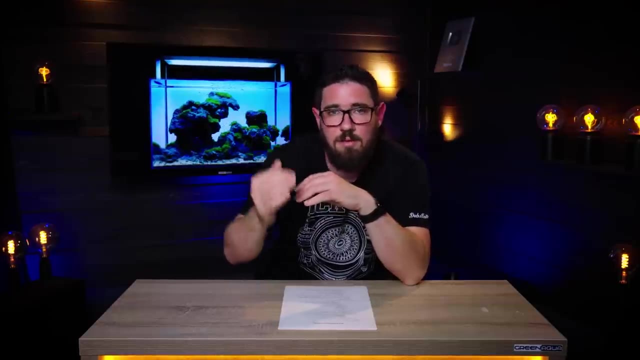 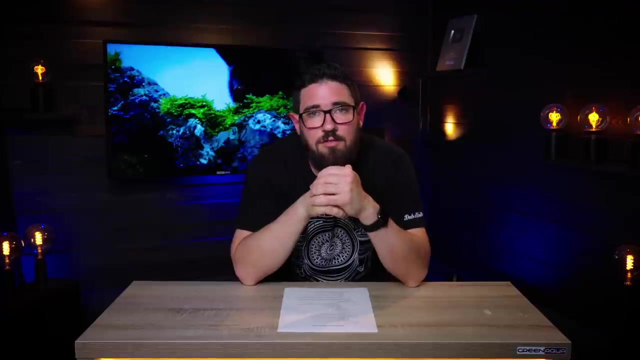 but have a CO2 controller which works like your room thermostat: If it goes above a certain level it turns on to drop it down. then it stops it, lets it go up. Yeah, that's it. It goes 0.2,- 0.3 levels of pH at a time. 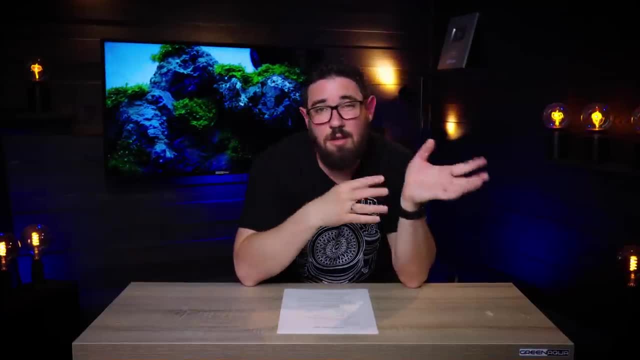 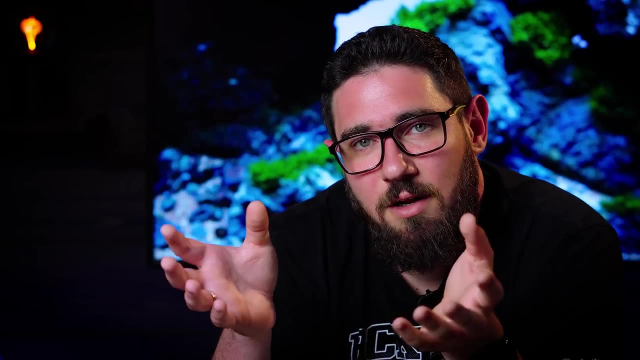 That's how you can keep it really, really stable, But it's not really for planted tanks. It's not a problem if you have something like this in a planted aquarium, but it's not required. So, all in all, it's really important to understand. 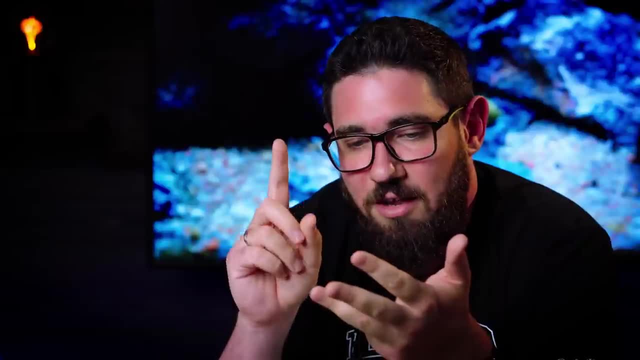 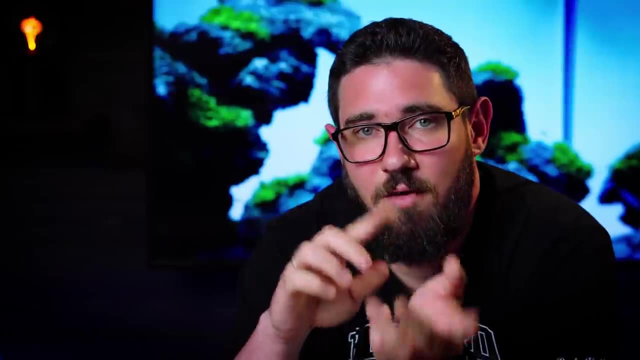 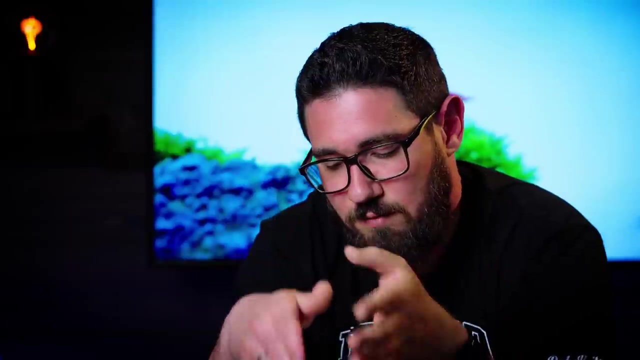 that TDS, GH, KH and pH are all connected, but you can't measure or convert one to the other. That's where a lot of people go wrong. So if you want to identify or have the amount of a certain type of 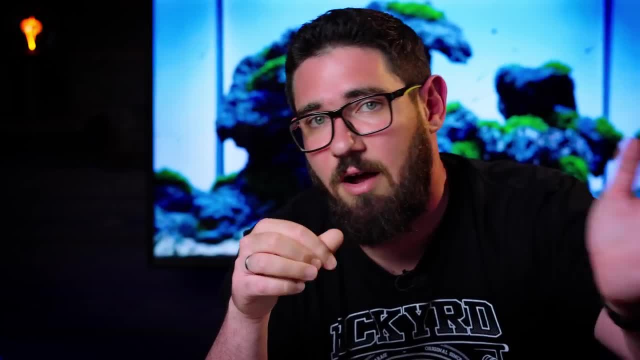 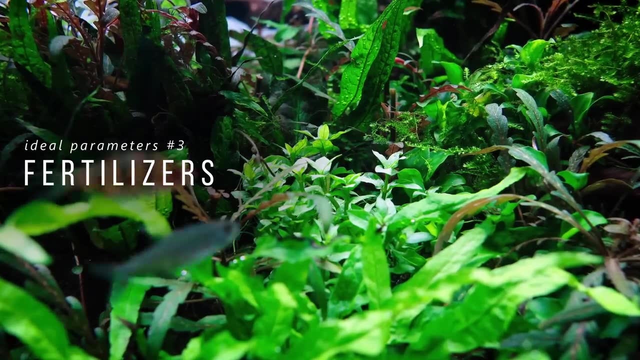 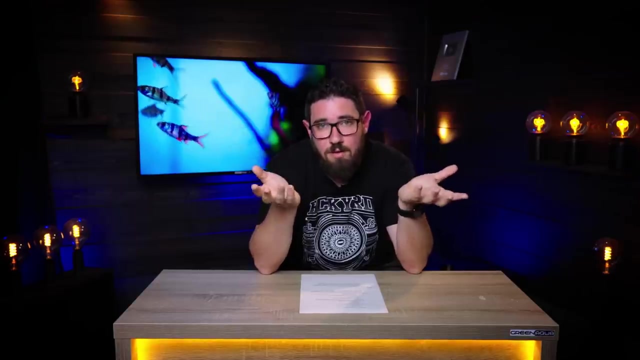 either of these in your water. measure that. Don't try to calculate GH from your TDS. It's not gonna work. Now let's switch to fertilizers. That's the other part we could measure. There is lean fertilization and estimative index. 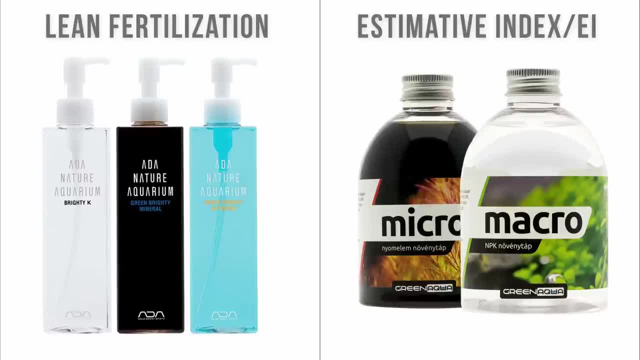 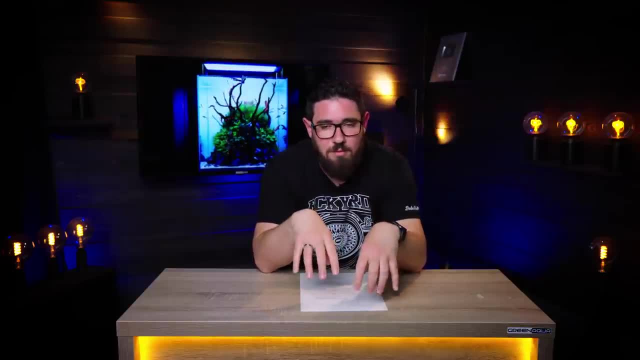 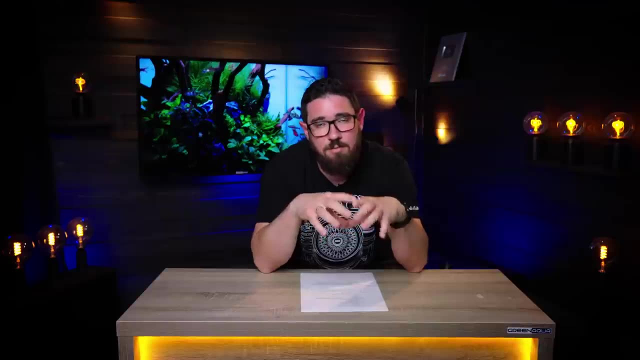 This is the two main ways of fertilizing an aquascape, and they differ a lot. The numbers I'm gonna tell you now are what you usually add during a whole week, So these are not the numbers you should measure in your aquarium. 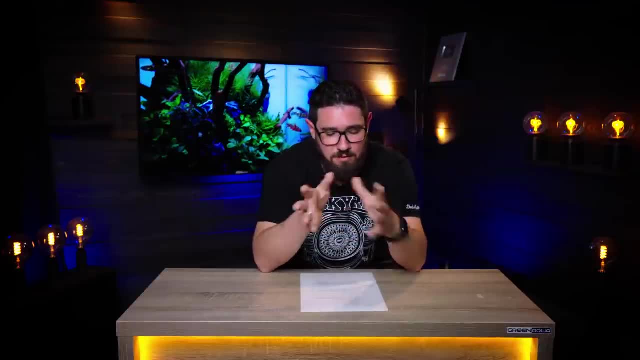 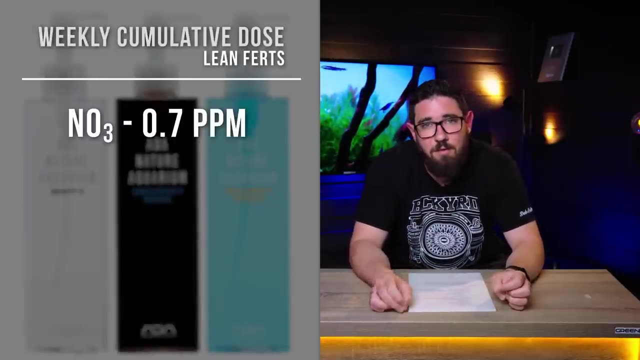 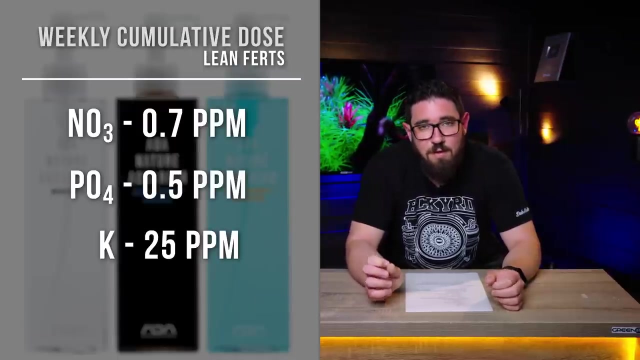 This is what you add in lean or EI fertilization. Let's start with the lean. You add about 0.7 ppm of nitrate in the tank, 0.5 ppm of phosphate, 25 ppm of potassium and 0.06 ppm of iron. 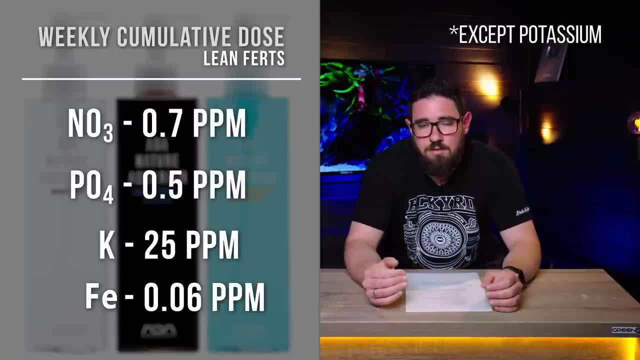 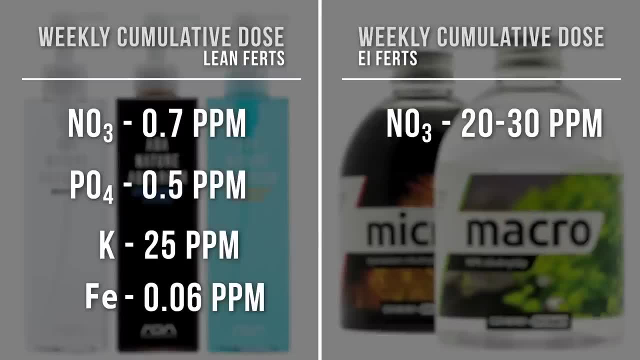 and other trace elements. So these are very, very low numbers and this is what you add during a whole week. In comparison with estimative index, you add 20-30 ppm of nitrate, 5-7 ppm of phosphate. 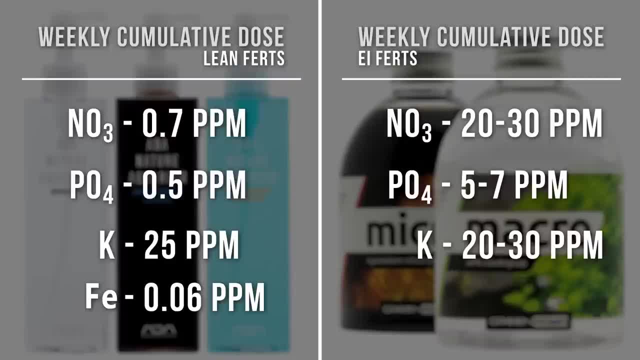 20-30 ppm of potassium, so almost the same level as with lean fertilization, and 0.5-1 ppm of iron and other trace elements. Again, this is what you add in a week's time, usually divided to days. 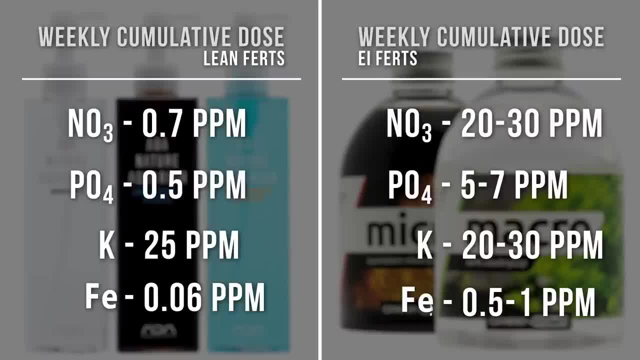 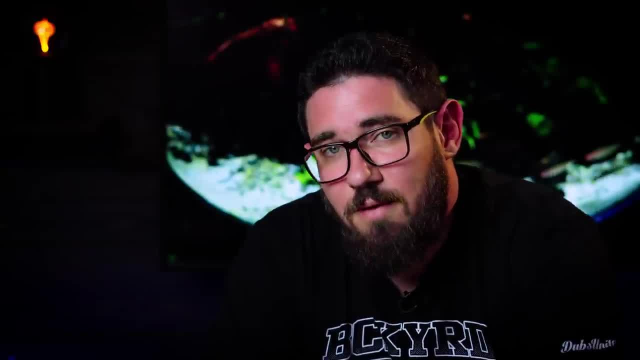 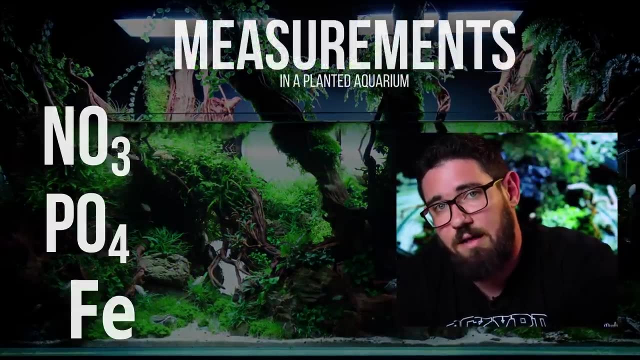 this is not what you should measure in your tank ever. These are not in correlation with what you have in the tank. What you should measure of each of these is the following: After dosing a fertilizer, you should have nitrates around 4-5 ppm at least. 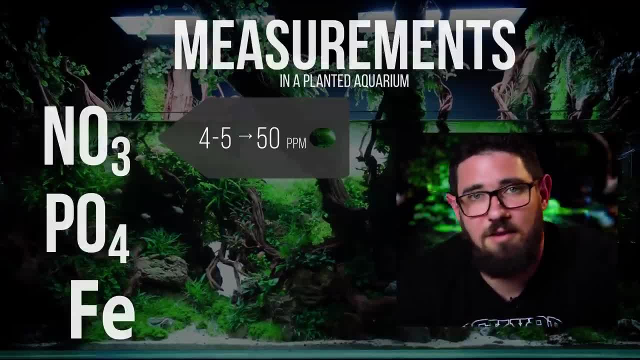 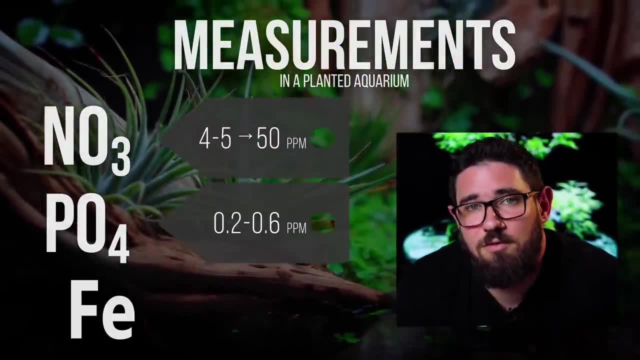 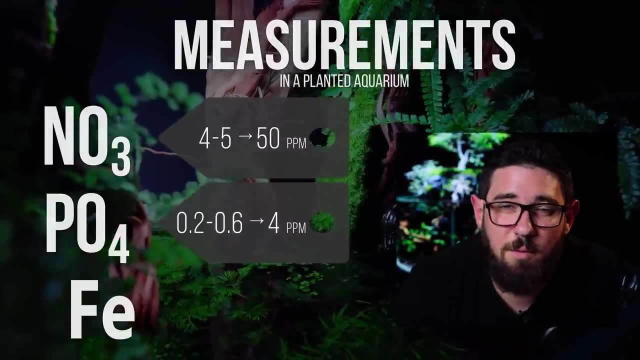 It can be 50.. Some people say it can be 150, and it's not a problem. Stick with 50.. Phosphates: you should measure 0.2-0.6 after adding your fertilizers. Again, it can be even 3-4 ppm. 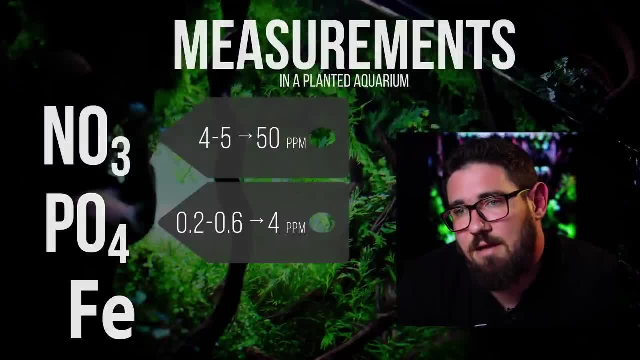 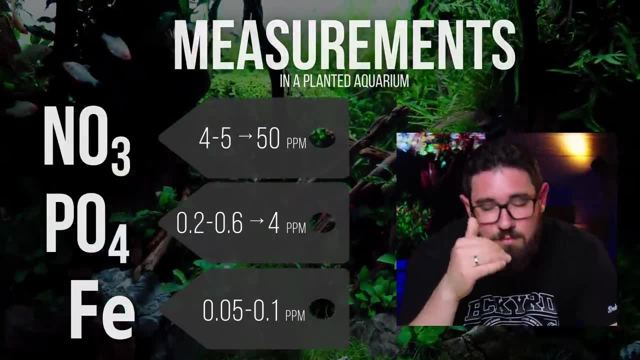 in an aquascape, but that level can already be toxic to shrimps, for example. For iron you can measure between 0.05-0.1 ppm And the rest again trace elements- you don't really measure separately. 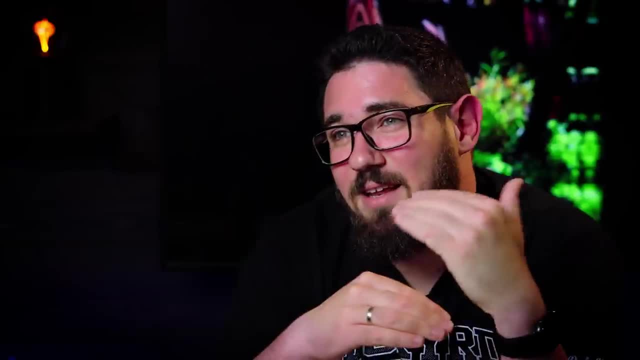 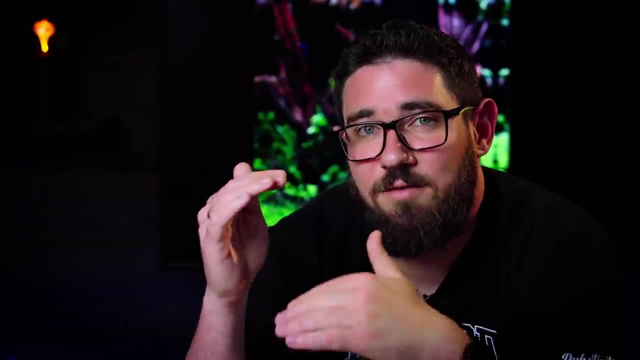 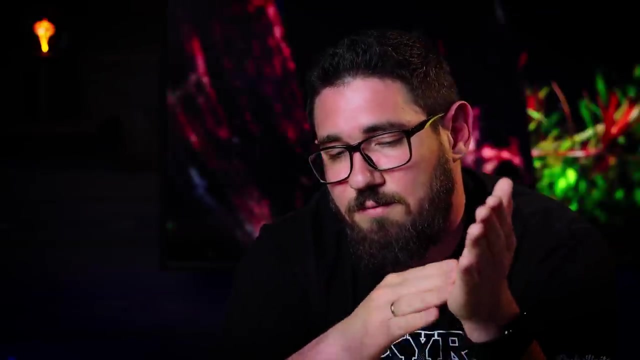 is the main indication of that. The more important thing than the actual levels is that a day after dosing- so before the next dose- you should still have some left of everything in the water. This means that there is always some fertilizer for your plants to take up. That's it. If something starts to build up really high in between fertilizing and even after water changes, that means that that type of fertilizer is not really taken up by your plants. The two elements that are mostly affected by this are phosphate and iron. 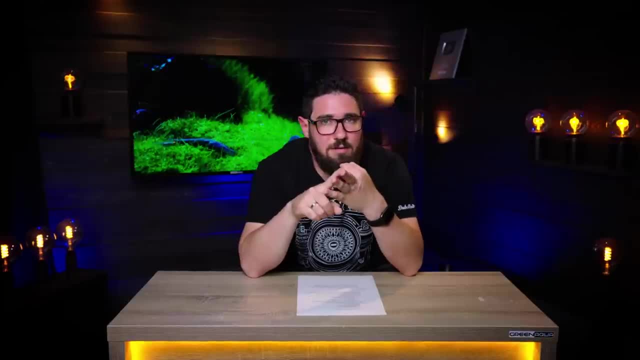 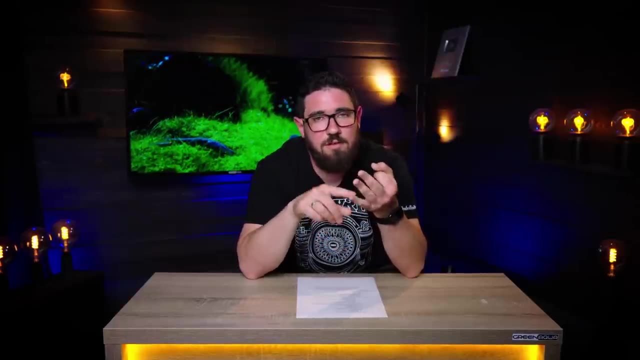 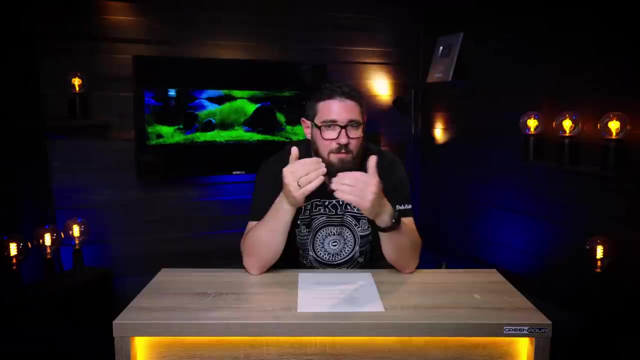 If you have low amounts of nitrate and potassium in your water and if you have low amount of CO2 or really crazy fluctuation of CO2, then phosphate and iron is difficult to take up for your plants. If you see that, for example, 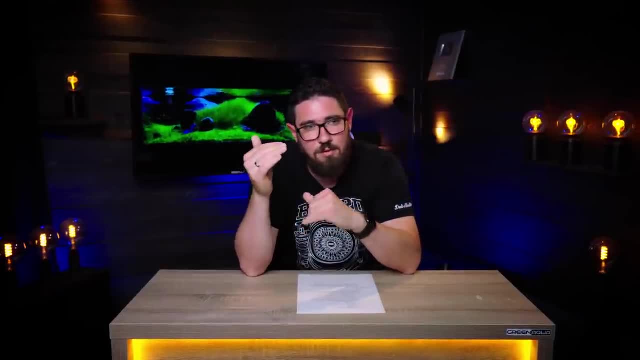 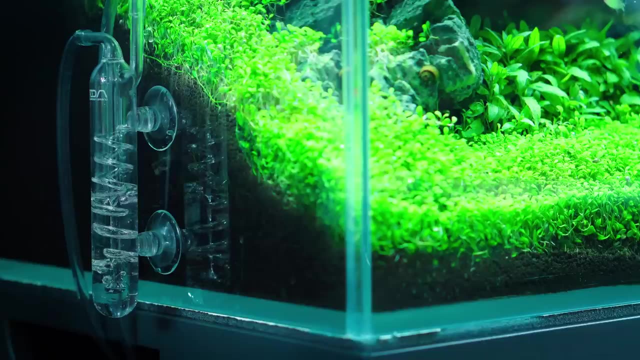 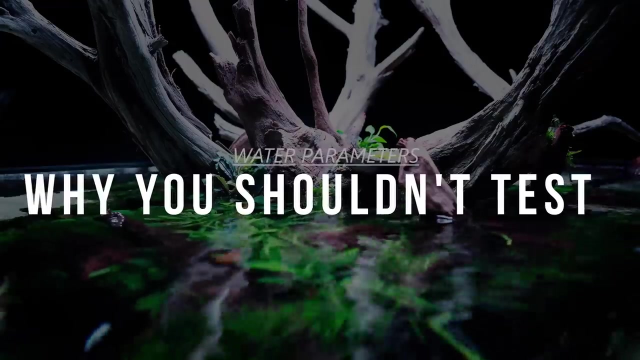 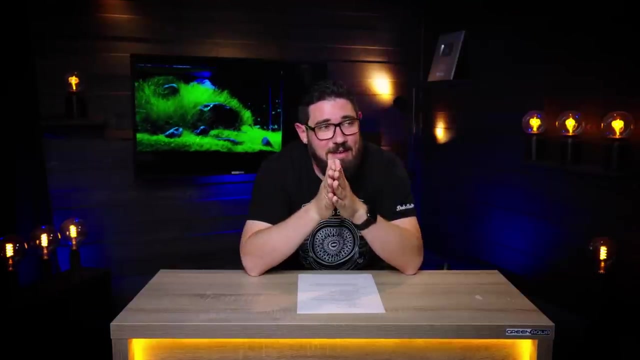 your phosphate is building up. you might be able to fix that by adding more nitrate or potassium, or probably the main issue is adjusting your CO2 to a better level and a more consistent level. And now, as I promised, let's talk about 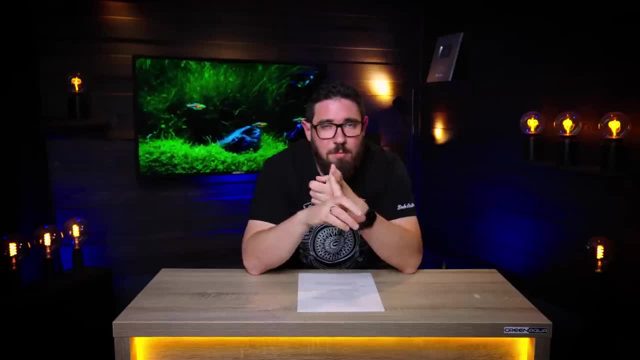 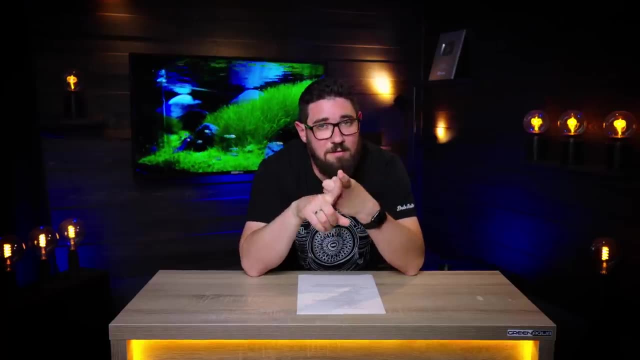 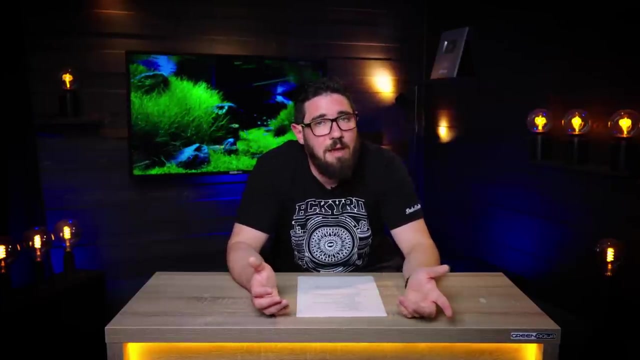 the main test and what the main problem is with most tests available. The biggest problem is that tests are made for regular aquariums, not aquascapes. So, for example, phosphate The level which is perfectly fine for us, it's like 1-2 ppm. 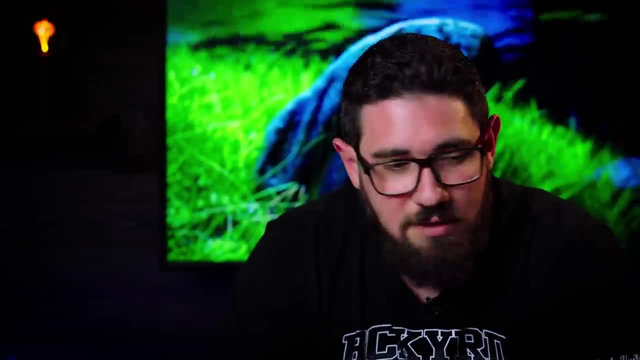 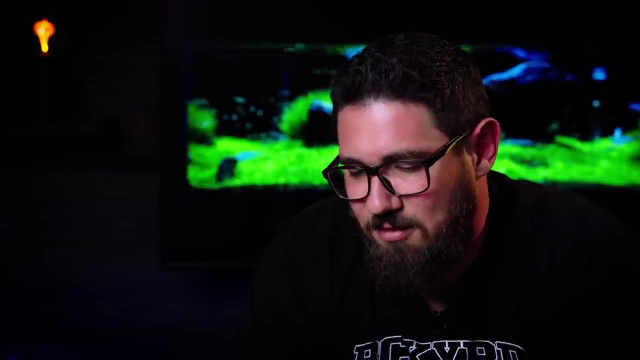 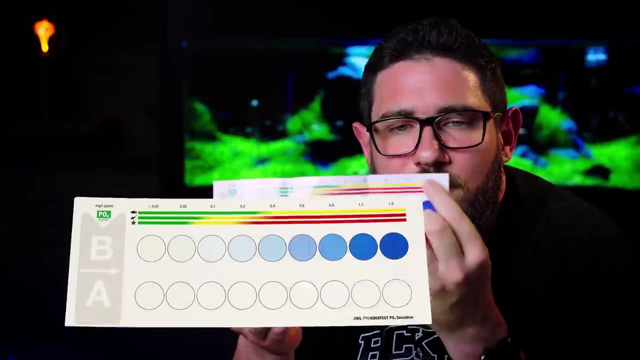 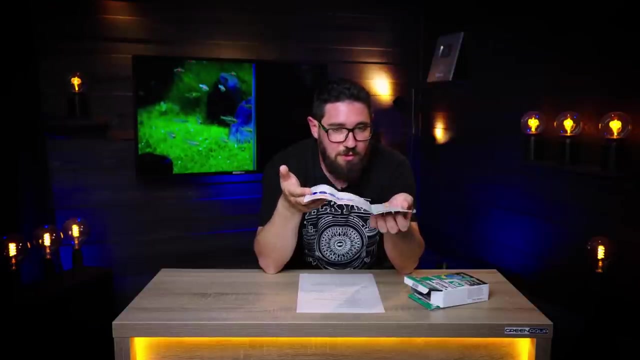 of phosphate that's shown really high and I think I need a phosphate test, The green one. Let's open this up. So this measures up to 1.8 ppm. We can go higher than that. A lot of people don't know this. 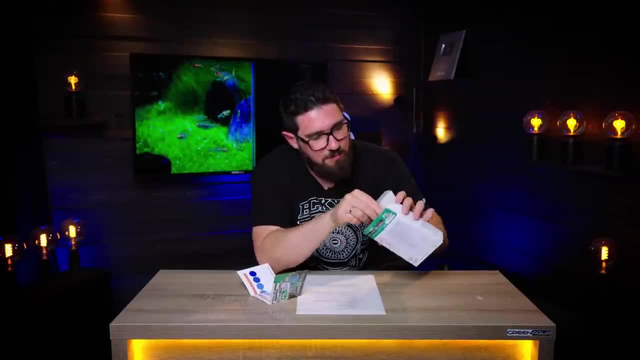 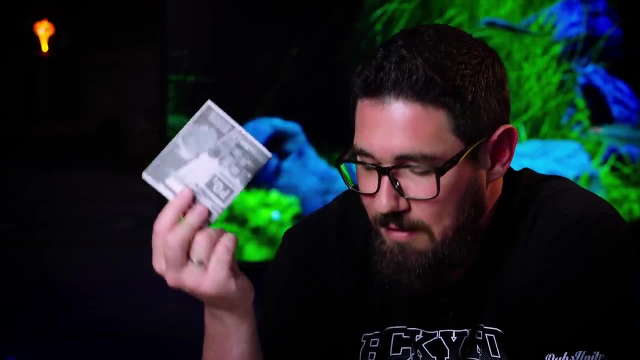 but you can actually dilute tests. So there are these things in most products. It's called a manual. This is what you throw out first time when you open it In case of tests. don't do that, because now I'm gonna look for it. 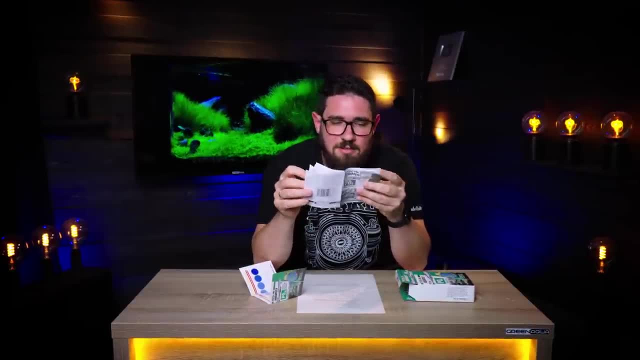 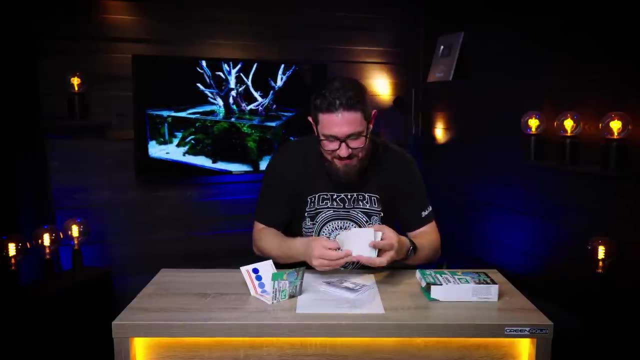 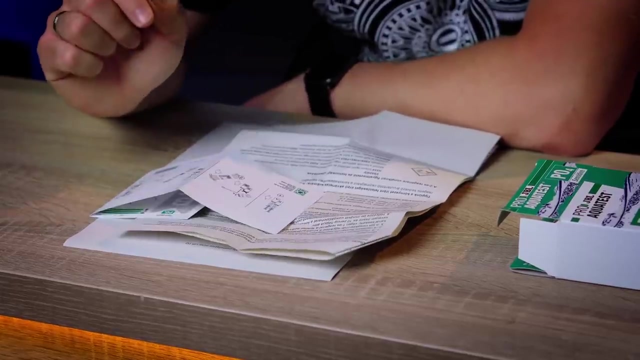 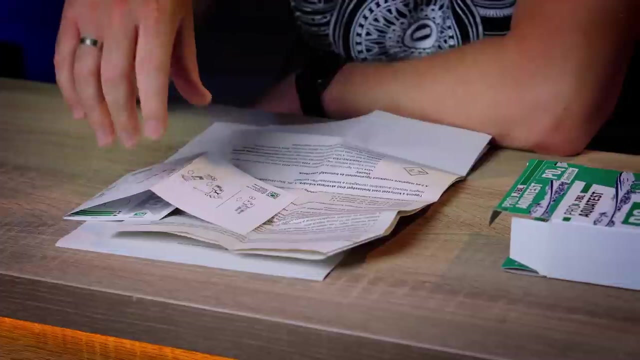 I just need to find a language that I understand- Italian. I'm learning Italian, but I'm not at that level to read this. You need 10 ml of aquarium water to do the test And you put the reagents into the aquarium water, But if you only use 5 ml of your aquarium water and add another 5 ml of distilled water or RO water to it and then do the whole process, then the result is twice of what you read. So in that case you read 1.2. 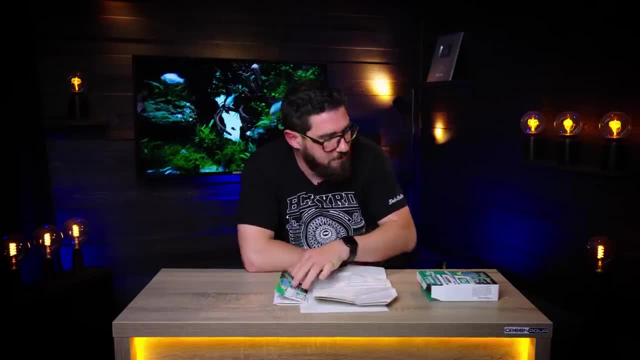 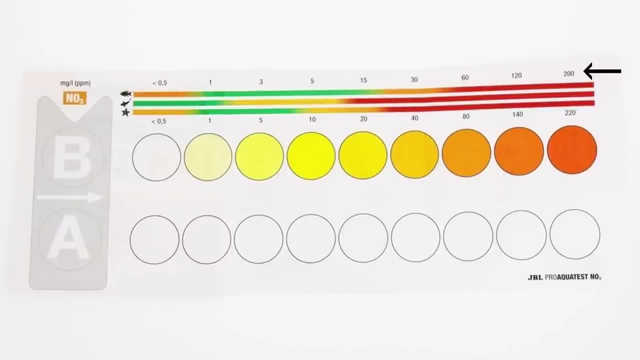 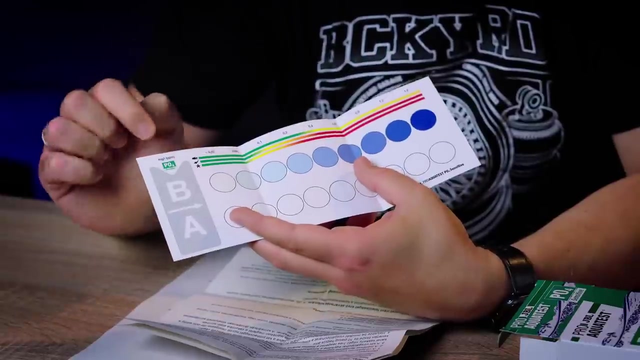 that actually means 2.4.. Also, I'm not gonna open another one, but for some tests the levels are different in freshwater and marine, and sometimes even in ponds. You need to make sure that you read the correct line On this one: the phosphate. 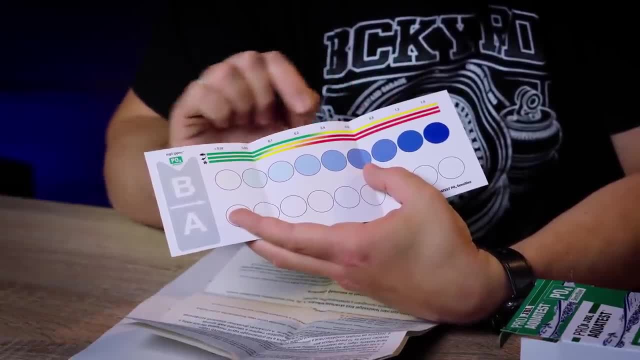 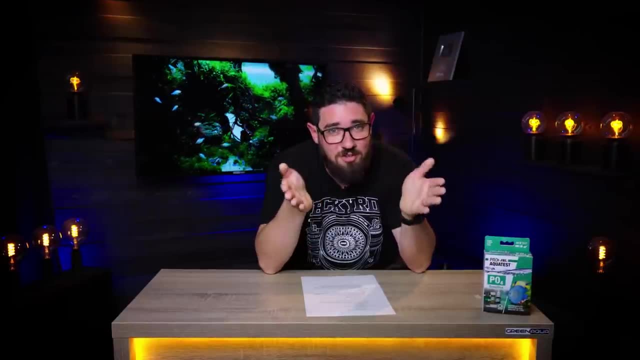 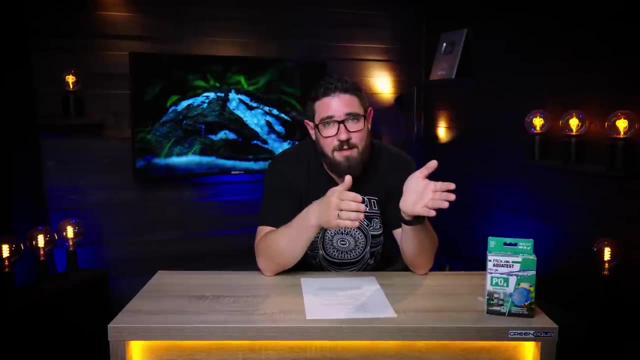 is just the sign of it being too high is what changes depending on the type of water? My main point why you shouldn't test is: we see this with a lot of clients. you have a tank that's running perfectly. You start measuring stuff. 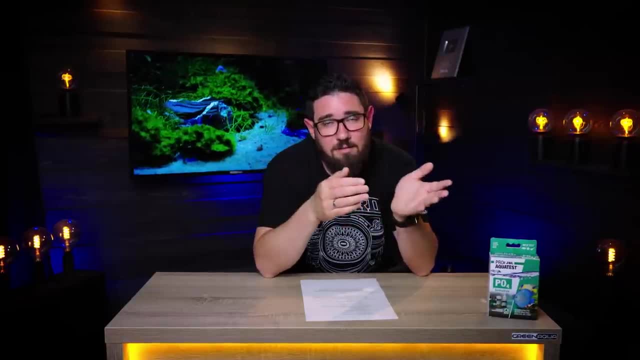 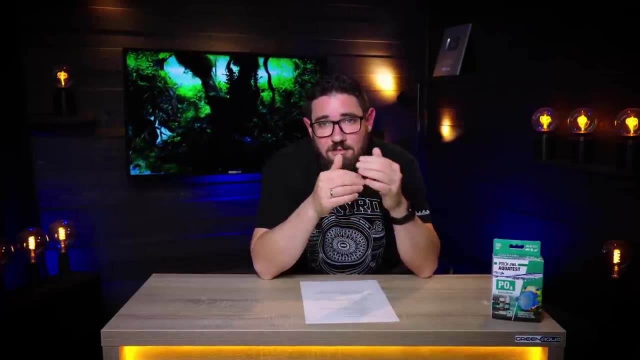 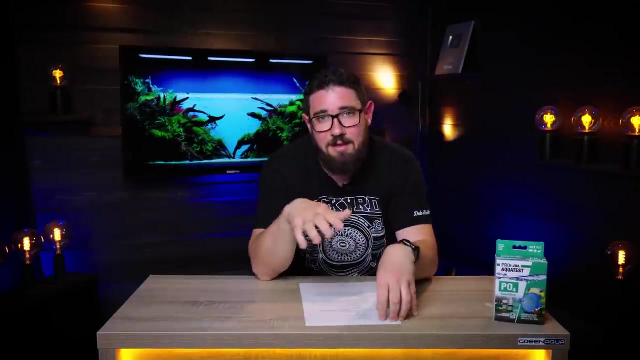 and the measurements say that your tank is not running perfectly. Please believe what you see and just let the tank go. Don't worry about measurements. They can be really off compared to anything that I've just mentioned and still it works fine. To prove this, I'm gonna head over to the showroom. 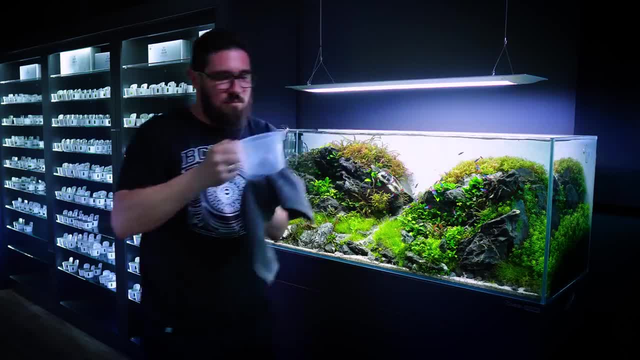 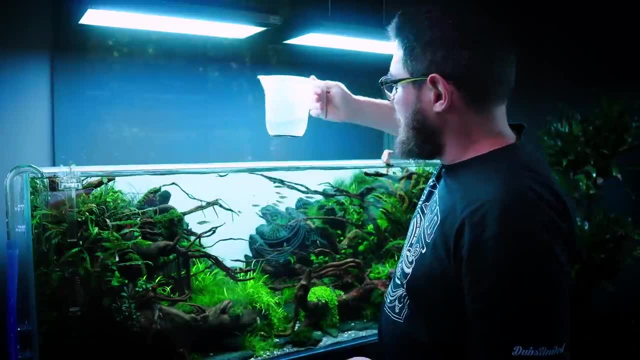 I'm gonna take water from two of our tanks which run perfectly, One of them with lean fertilization and ADA in this example, and one on estimative index, the green aqua fertilization, and we're gonna see what we measure. 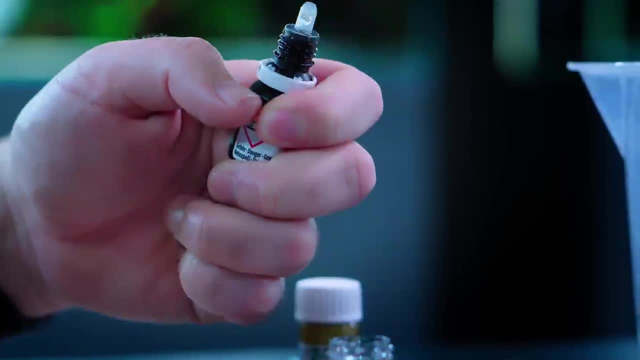 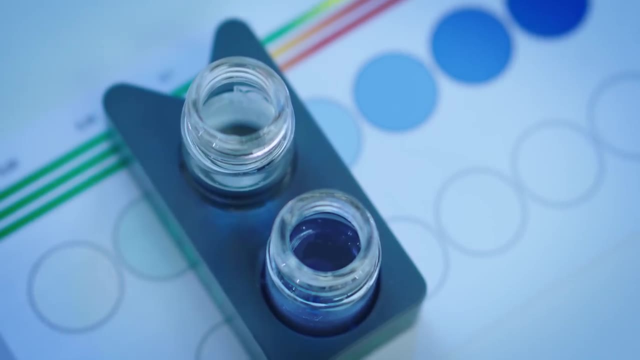 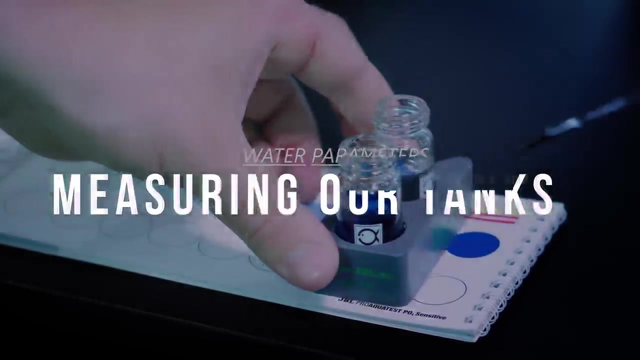 I'm sure that we're gonna have some stuff that are way off what's recommended or what we would aim for if we would really care about this, and that proves that it's not a problem. Let's see. So I have the measurements of the two. 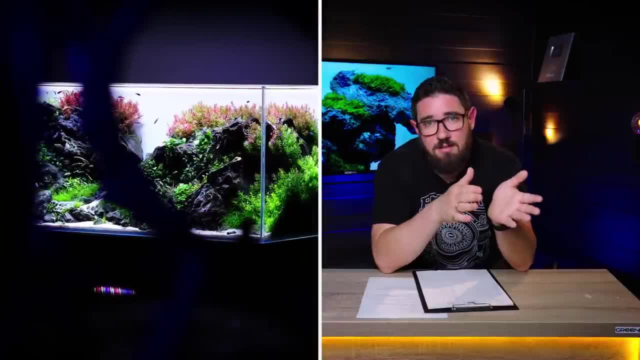 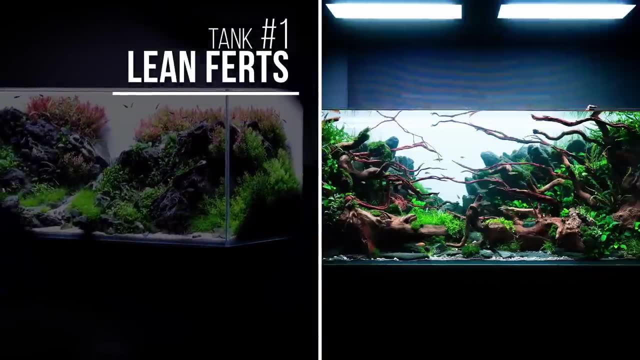 tanks. One of them is Balazs Brazilian Scape. It's running on ADA fertilizers And the other one is, yeah, again Balazs Scape, the other 120P which is running on estimative index green aqua fertilizers. 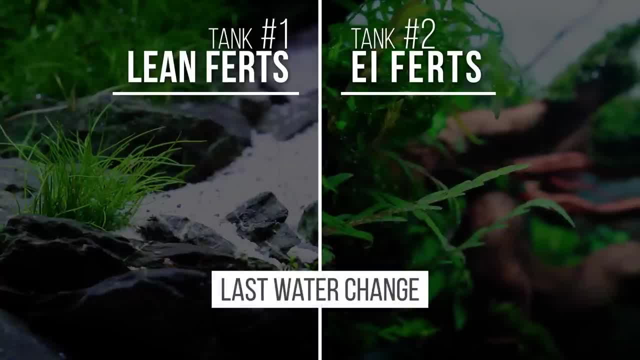 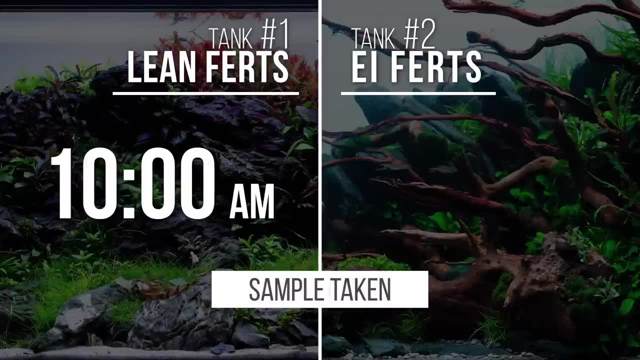 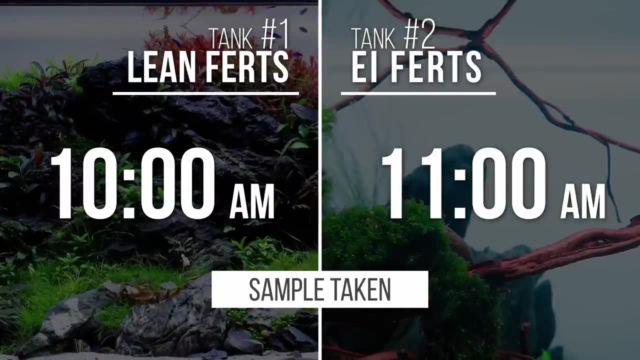 Both tanks have had their water changed three days ago and the water has been taken out of them at 10 and 11 AM, so one and two hours after the lights went on and three and four hours after CO2 has been turned on. All these factor in 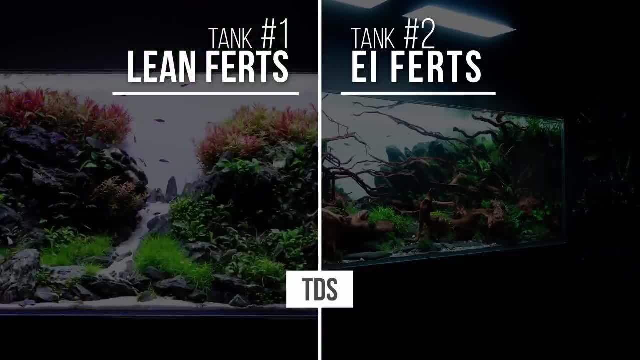 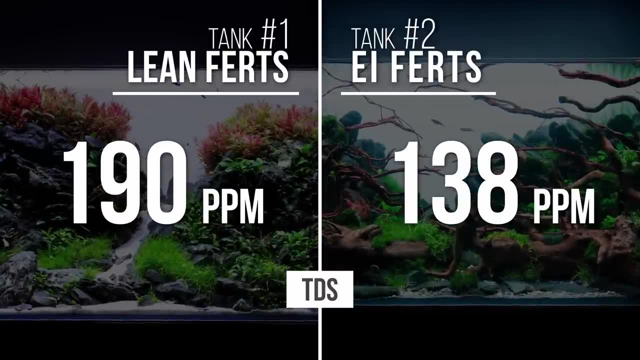 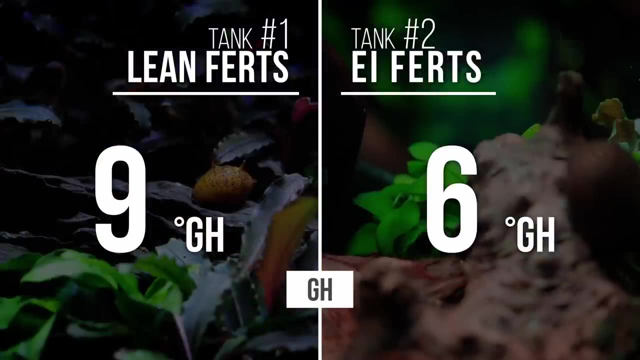 into the measurements. Let's start with TDS. The Brazilian has a TDS of 190.. The other one is 138.. GH is 9 on the Brazilian and 6 on the other one. KH is 6 on the Brazilian and 2. 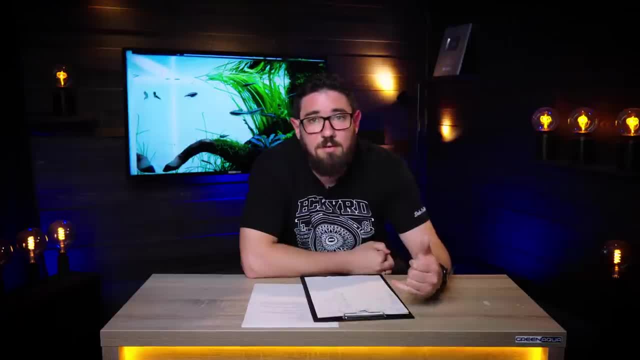 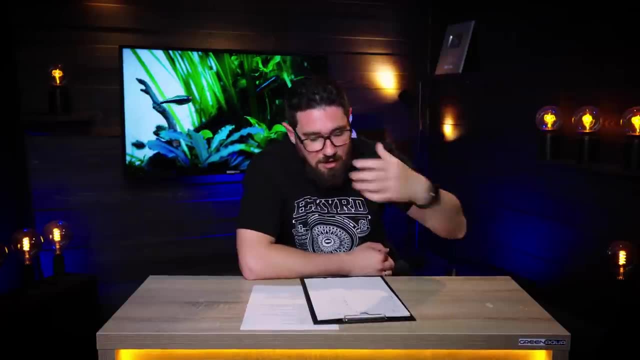 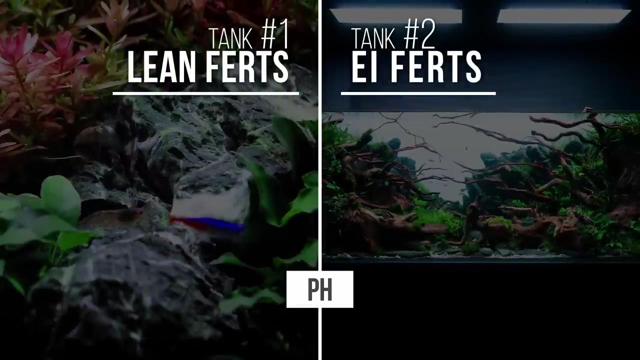 on the other one. All this already shows how the serious tones in the Brazilian Scape raise at TDS, GH, KH, everything. So you can see that change quite easily. This is after three days pH. The first one is 6.8, the other one is. 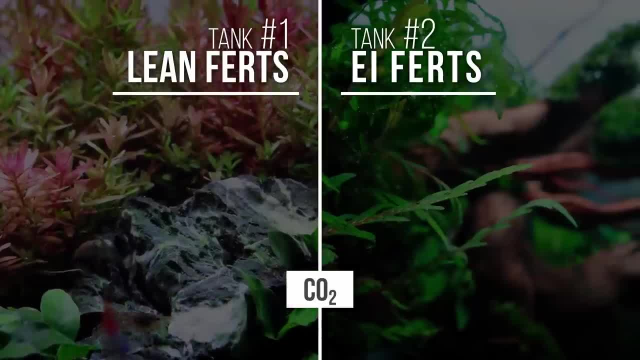 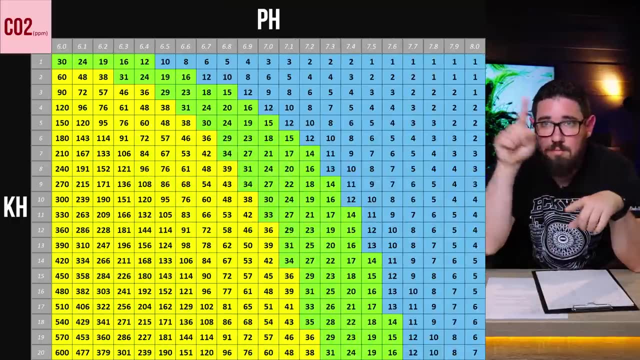 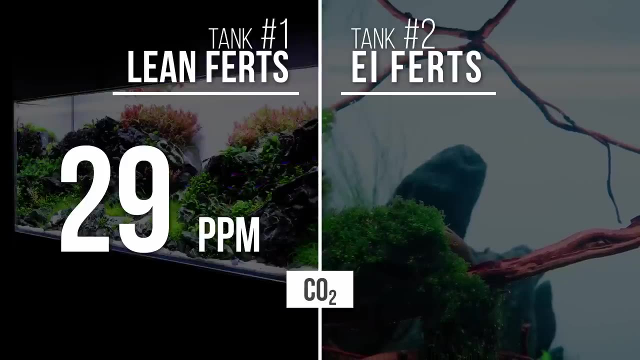 6.3. CO2 measurements. This is calculated from the ratio of KH and pH. There are these charts where you can see both of them, and then it says CO2 in ppm. So it's 29 ppm in the Brazilian and 31 ppm in the. 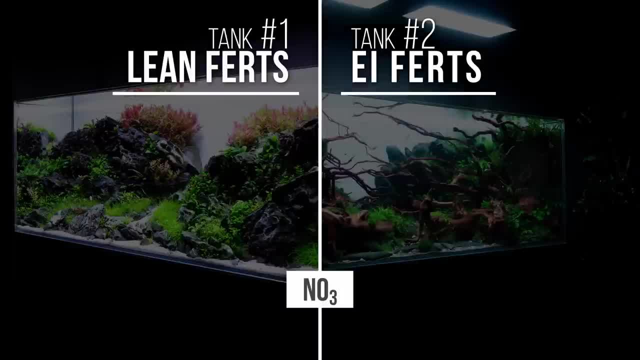 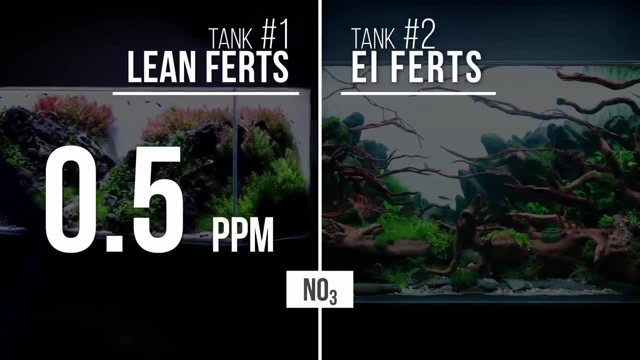 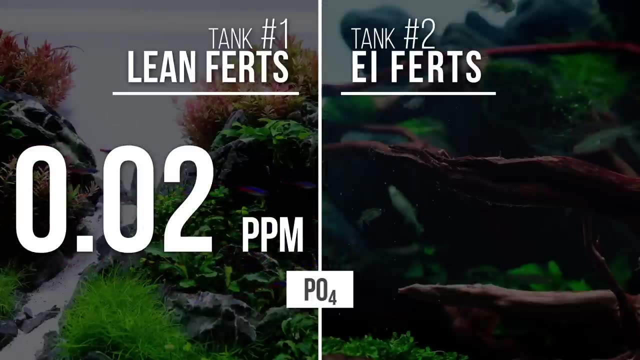 Wooden Scape Nitrates: With ADA, it's 0.5 ppm. With the Estimative Index it's 20 ppm. Phosphate 0.02 with ADA and 10 ppm with the EI. fertilization Potassium 13. 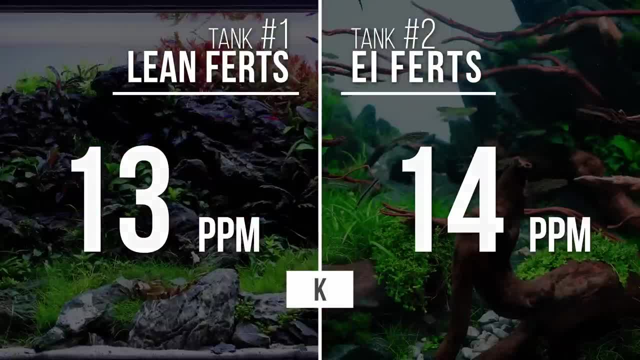 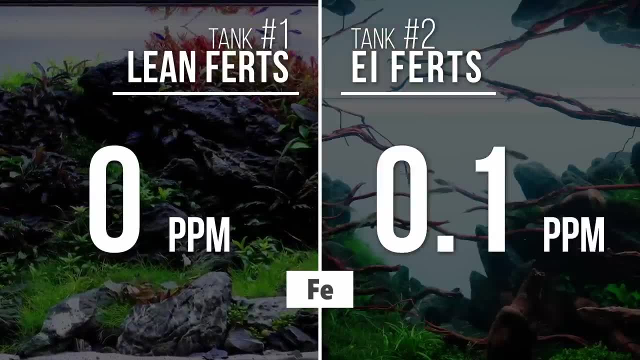 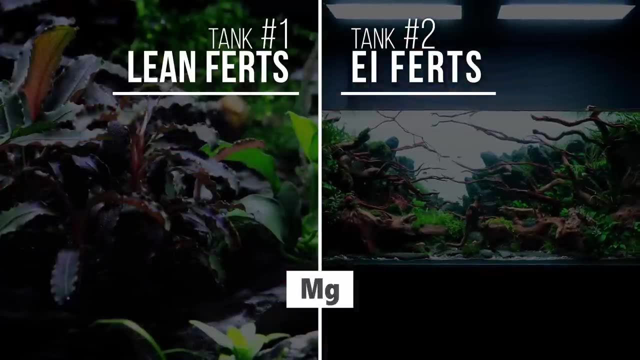 and 14, so almost the same. Iron is 0. Basically unmeasurable in the ADA one And 0.1 in the EI tank. And then we have magnesium as well, which we don't really measure. but now here it is, It's 6. 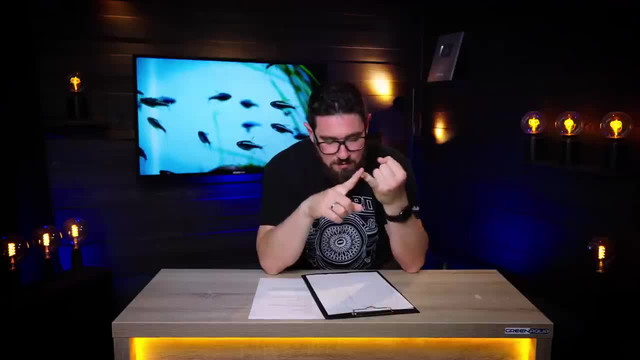 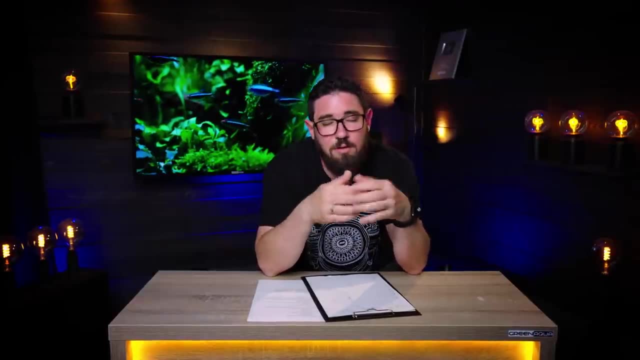 and 8.. What we can see here is, first of all, big difference in the two types of fertilization. That's what we expect, especially visible on the nitrates and phosphate. Let's compare this with the recommended measurements to see. 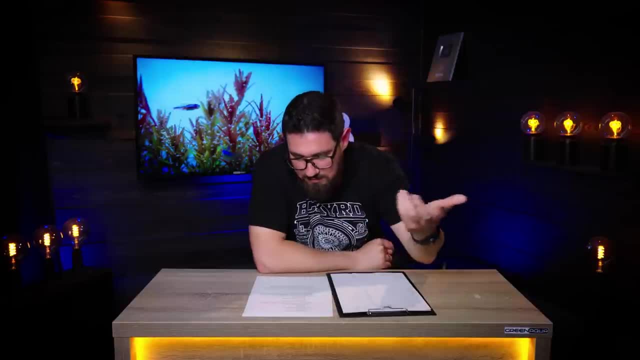 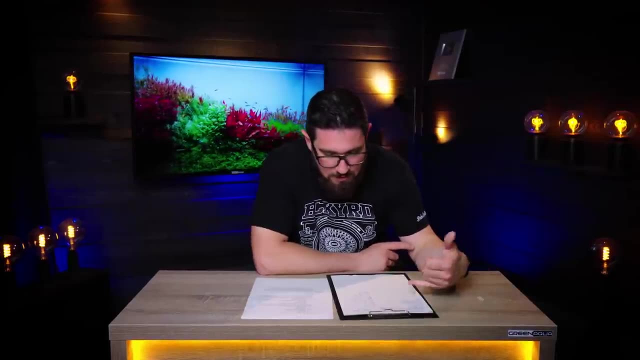 if they're okay or not. For example, nitrates. I said 4 to 5 ppm, but it's fine up to 50. Well, in the ADA one it's lower than recommended. In the EI one it's higher. 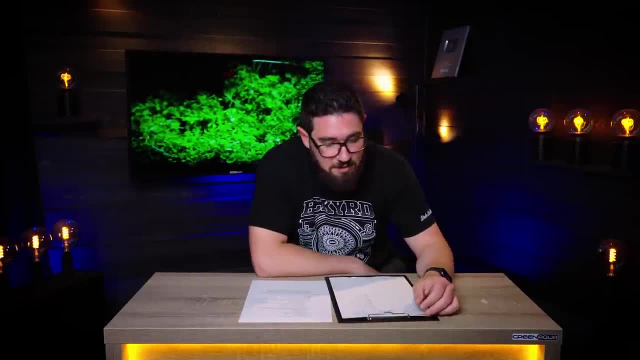 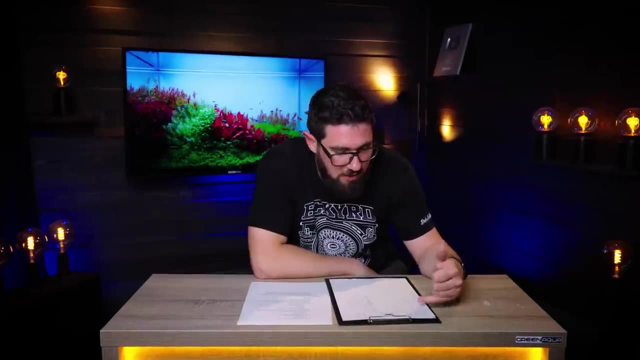 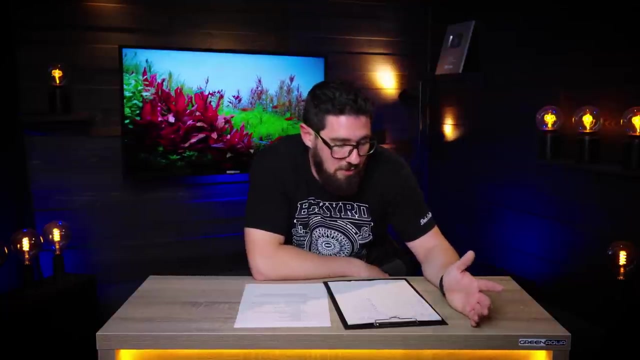 than recommended. Still, the tanks are looking fine and running fine. Same goes for GH, KH. The GH and KH in the Brazilian is quite high compared to what we usually aim for, But that's because of the serious stones and we don't have any. 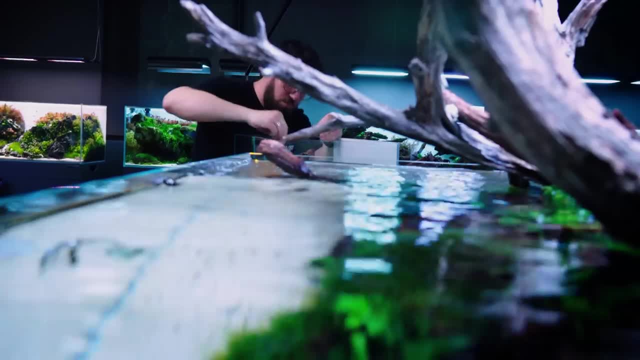 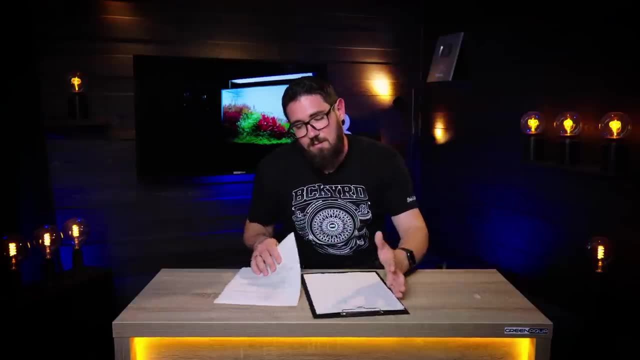 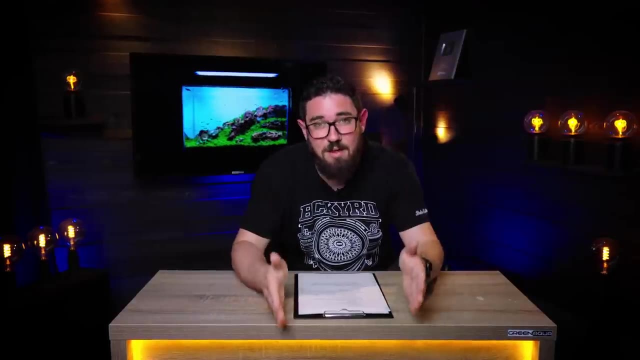 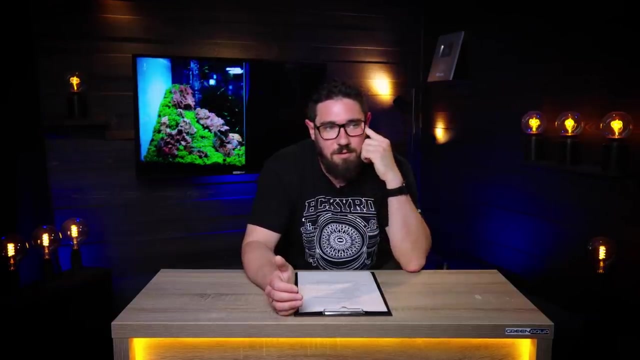 problems. pH is quite different as well. This is what my conclusion is with this video, Which I mentioned earlier as well: Don't measure unless you need to. If there's a problem, ask for help from someone who knows his stuff, Don't just go. 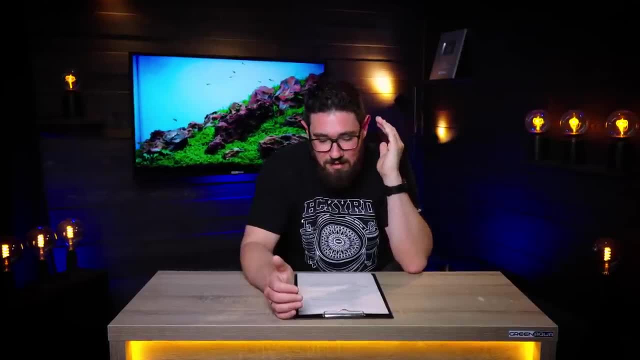 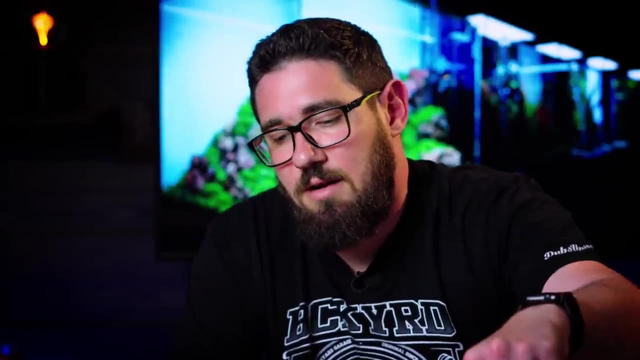 online, because you're gonna see a lot of different stuff and that's gonna be really confusing And if you make any adjustments, if you have a problem in your aquarium and you make adjustments, let it go for 2 or 3 weeks before you try. 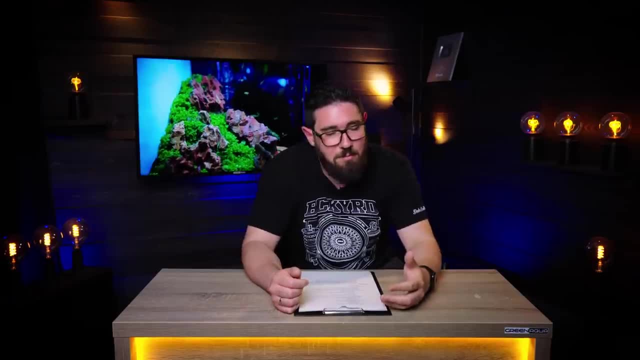 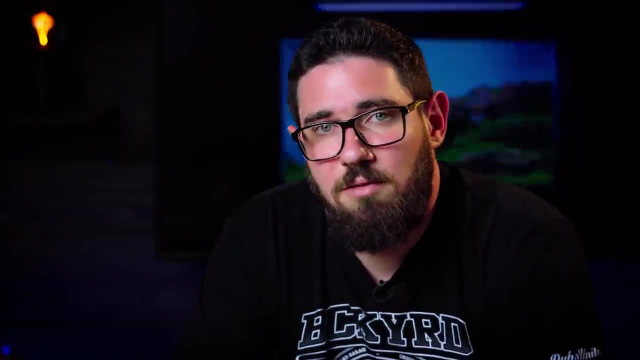 to decide if it's better or worse. This is a big problem as well in aquascaping. You have a problem, someone suggests you a solution, you try it and you expect it to work like magic in 2 days And nothing happens. 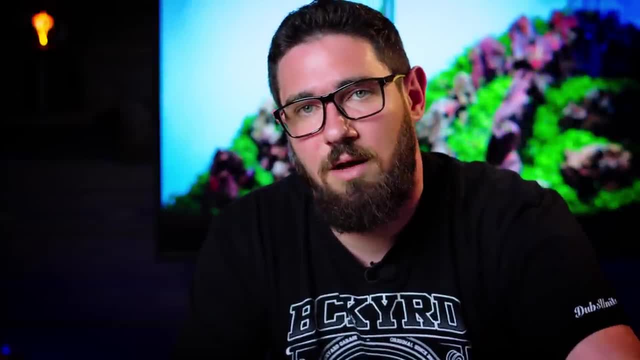 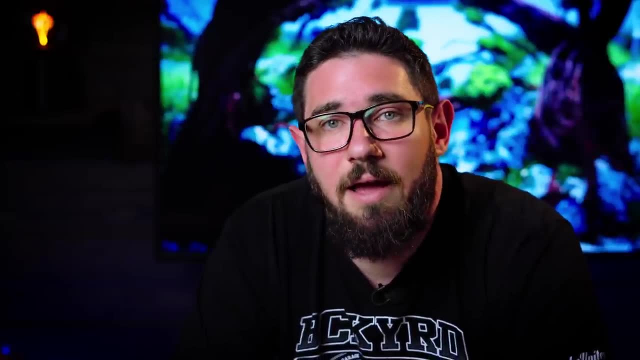 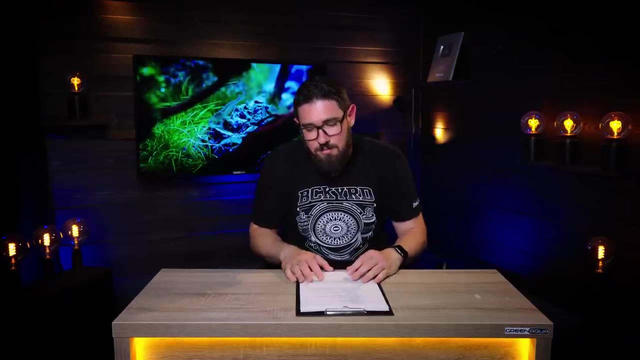 and you go to the next thing. Then you're never gonna know what actually solved your problem Or, even worse, you might get it really wrong and you just destroy your tank. Be patient, as always, And to all this measurement stuff and fertilization. 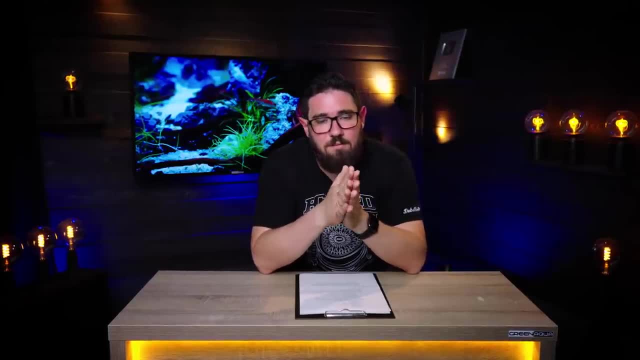 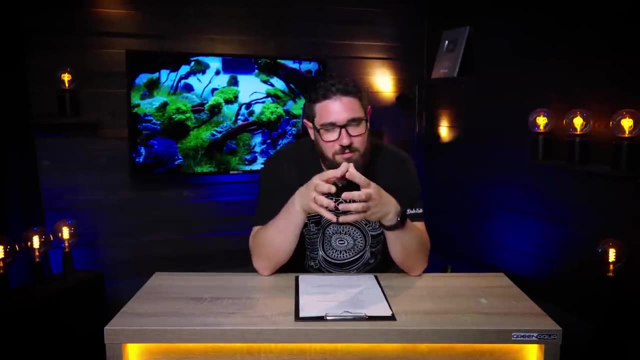 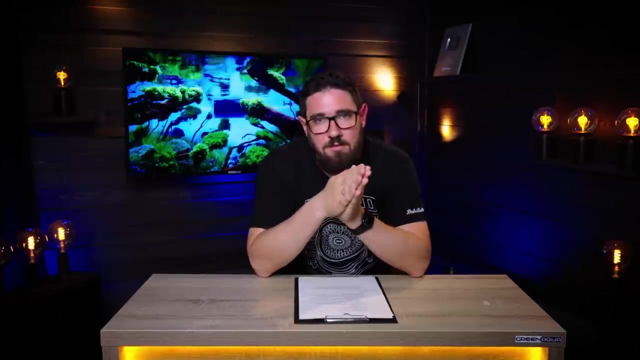 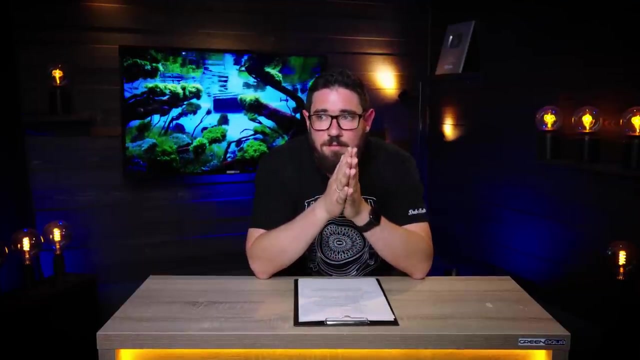 if you have a kind of fertilizer that someone designed and tested and it works well for a lot of people, then in most cases the problem is not with the fertilizer and not with these measurements that we've talked through. It's most likely your CO2 system. 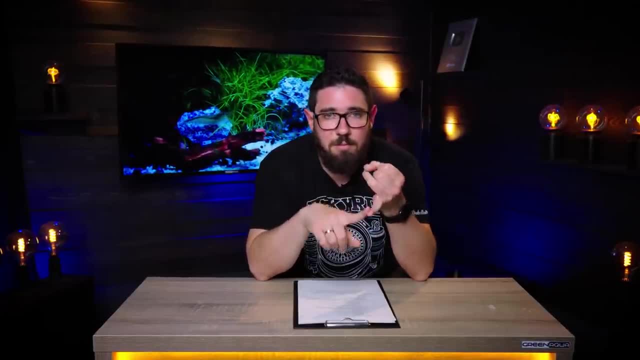 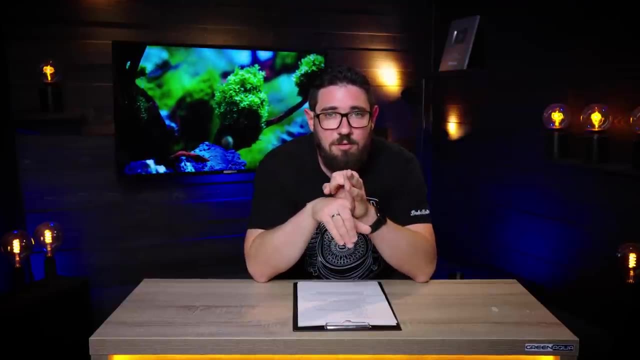 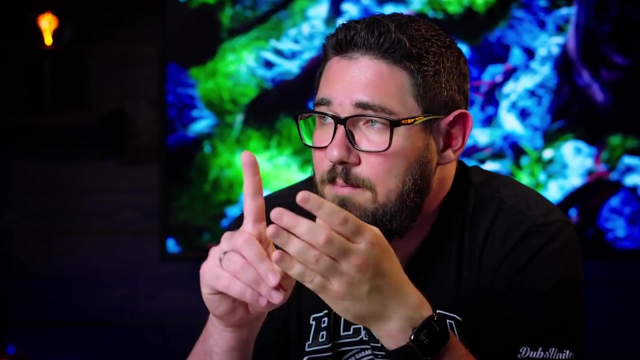 your CO2 levels are fluctuating. not properly set water temperature- we always talk about this- High water temperature can do crazy things to your tank and your plants and algae and everything else. Improper filtration, improper maintenance, lack of water changes. 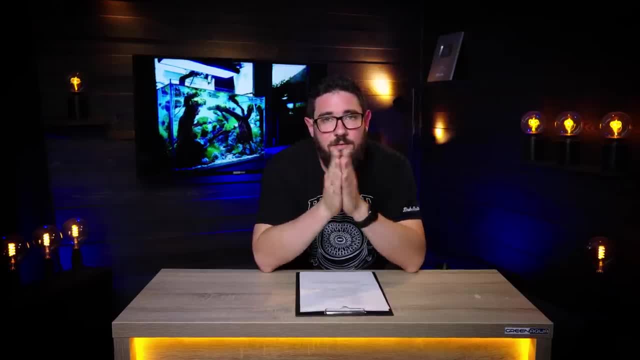 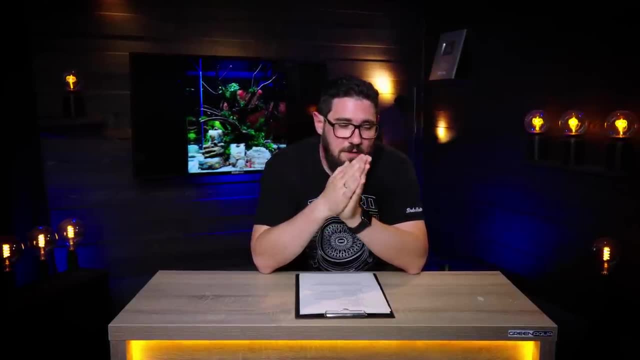 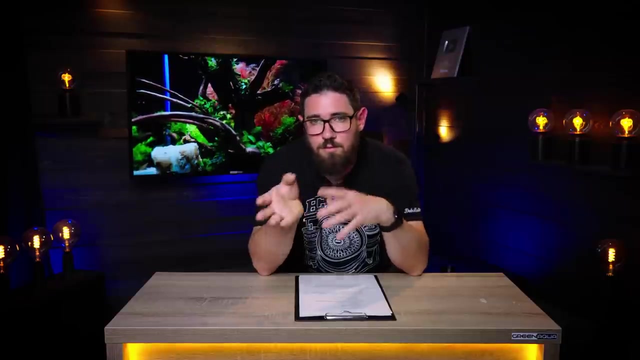 and so on. These are the things where you find the issue 90% of the time, And if you start measuring stuff and if you start trying to solve your problems by changing fertilizers or adding stuff to your current fertilizing lineup, it usually 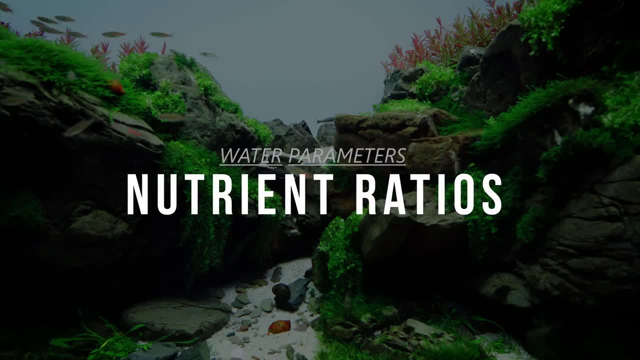 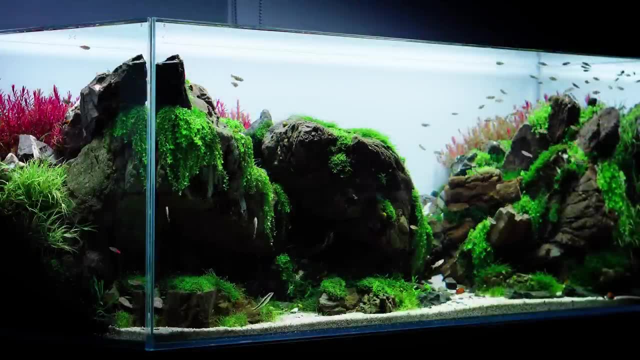 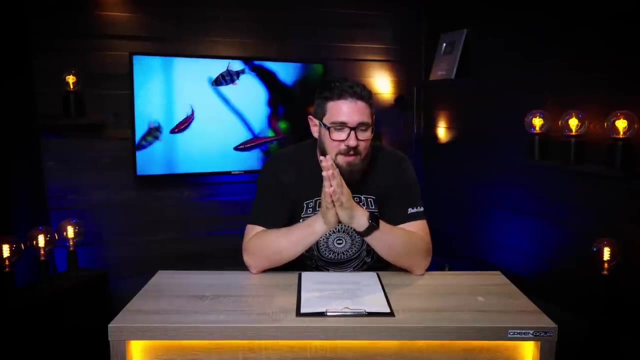 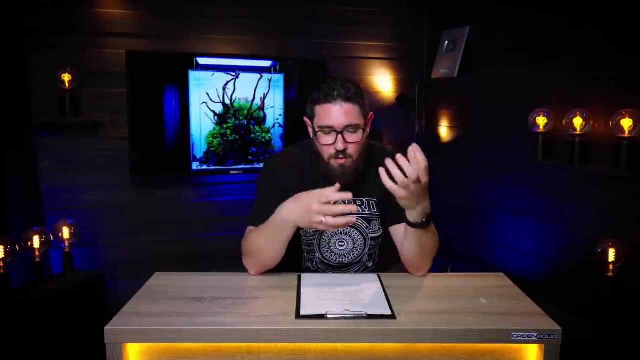 goes into an even worse place. There's something I didn't talk about, and probably some of you are missing it: The ratios of nutrients. This is a thing that a lot of people consider important, and they say that the ratio of all the separate elements is important in. 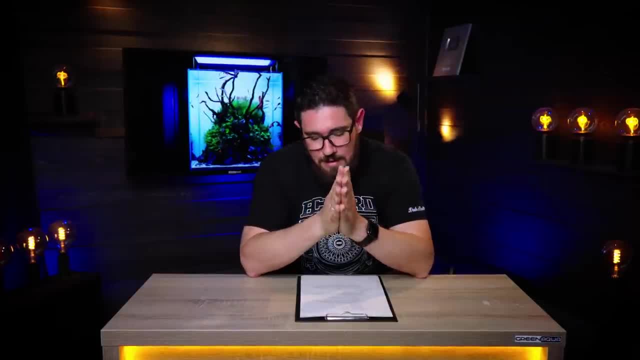 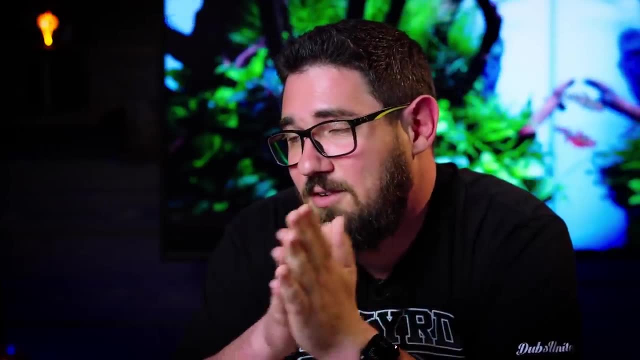 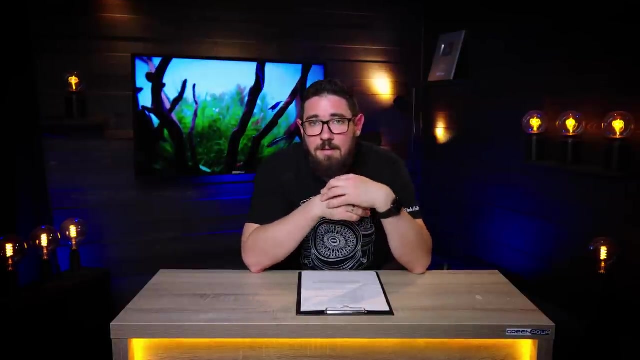 the process of taking up nutrients by the plants? In our experience it's not. This is a long time debate. It's going to go on forever and I don't want you to choose sides. I want you to experiment If you feel like that's. 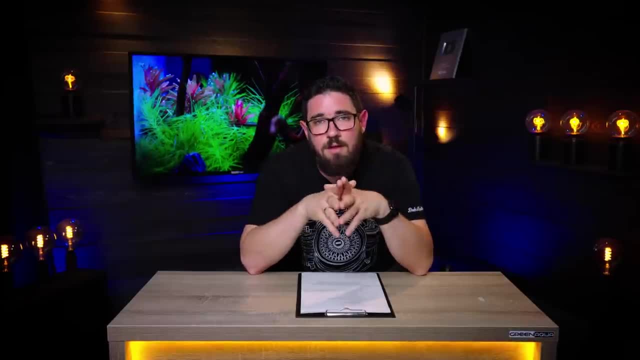 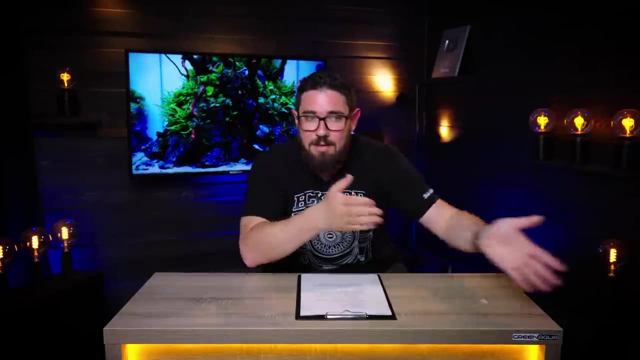 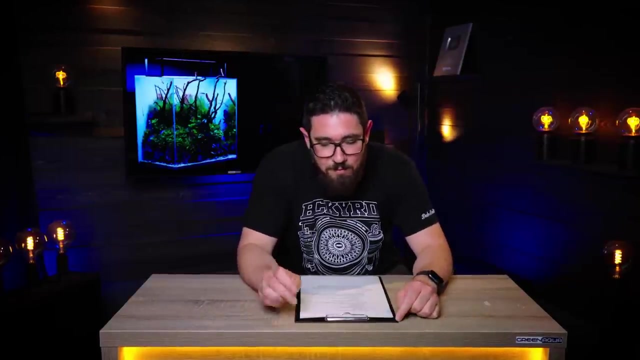 something that's more understandable for you and you think it has some merit, then go for it. You can keep ratios of nutrients. It's not going to be a problem if you keep certain ratios of nutrients. We just believe that it's not as important as some people think. 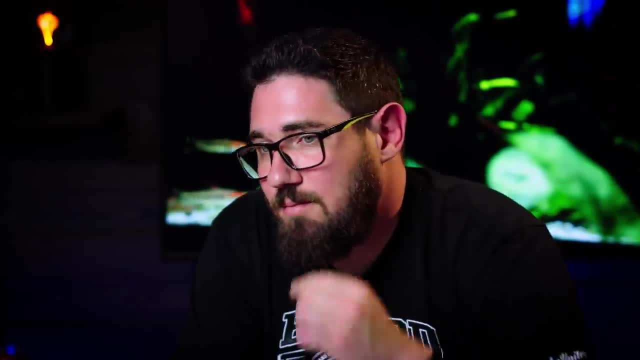 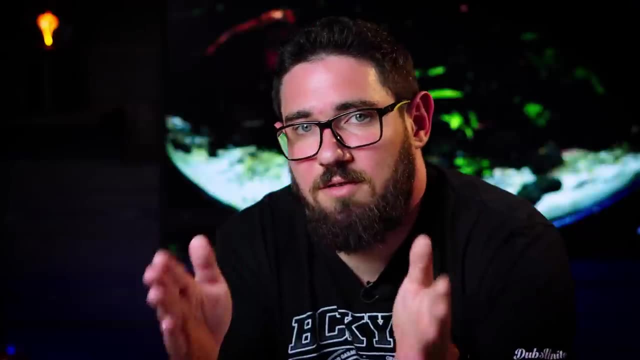 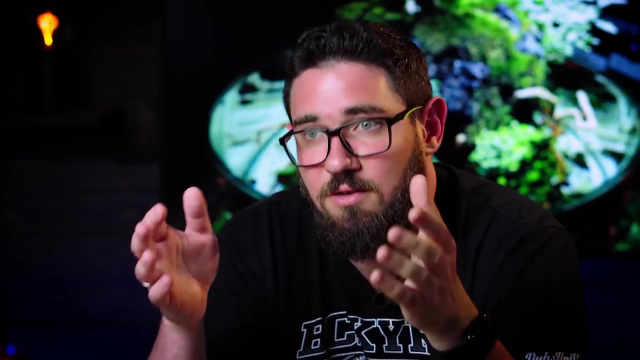 That's why I didn't want to go into it. You can go online and find ratios that some people keep. Go for it, Try it. The only thing is, if you start to escape, choose a type of fertilization and choose a type of fertilizer, a certain brand. and stick with it. Changing fertilizers during the lifetime of a certain setup is really stressful for the plants. That's something we don't really recommend If you want to try both ways, even like lean fertilization and EI, or keeping ratios or not. 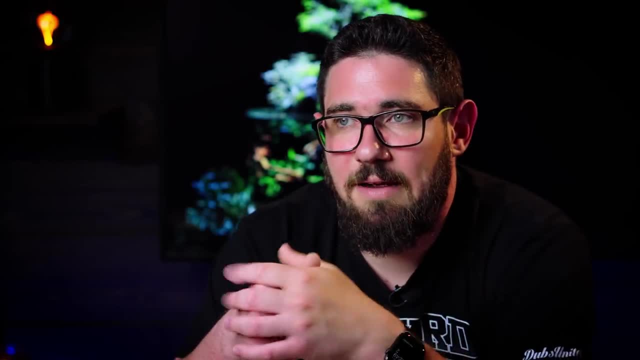 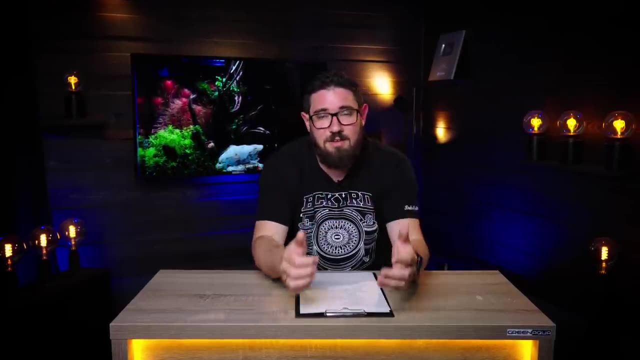 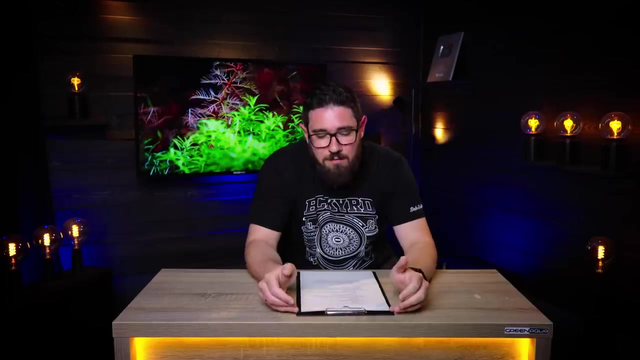 you should do this in separate tanks. This is my point of view on this. This is our experience with fertilization and testing. There's a lot of debate about everything that I've just talked you through. You're going to find really different opinions. 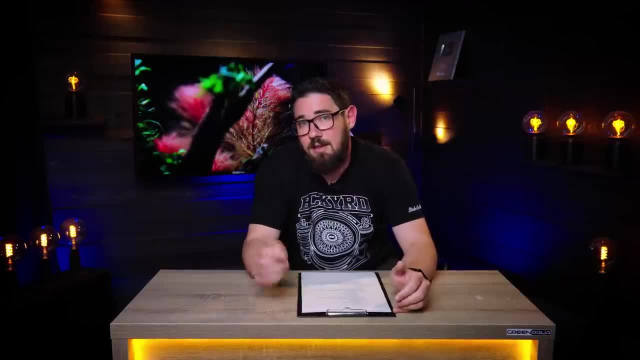 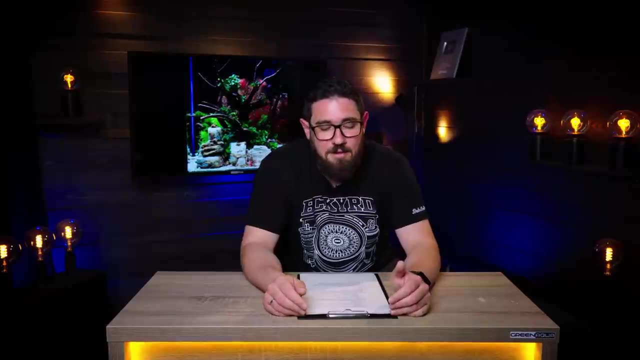 I'm sure that we're going to have a lot of different opinions in the comments section below and please, I encourage you to give your opinion about all this. Just please, keep it civil. I think we're never going to see who's right. 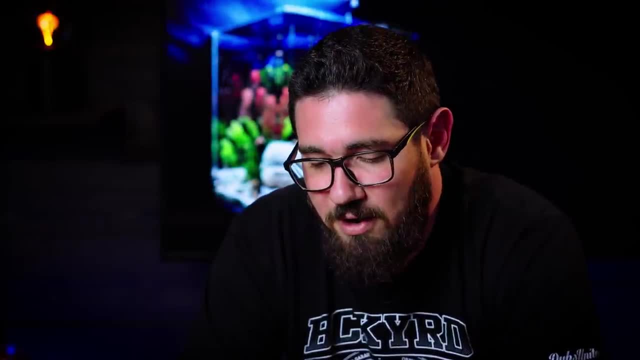 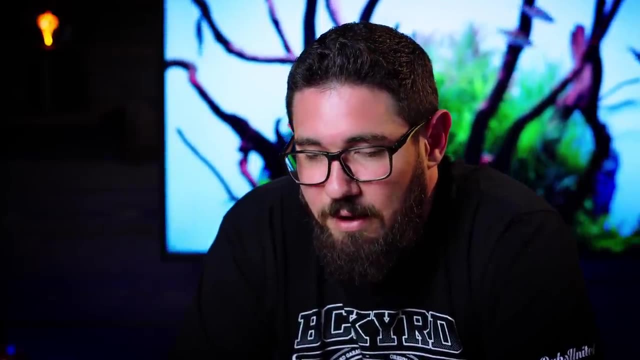 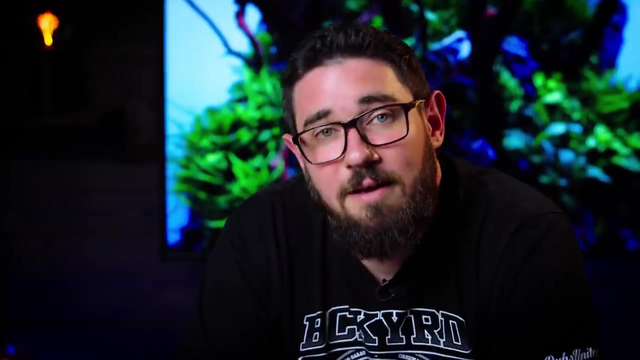 It's a debate that's going to go on as long as we have aquascaping And it's part of our hobby. That's it. What I hope is that everyone finds the way that's working for them, And that's what's important.